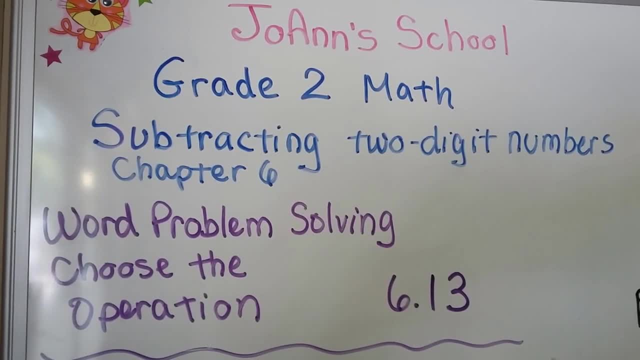 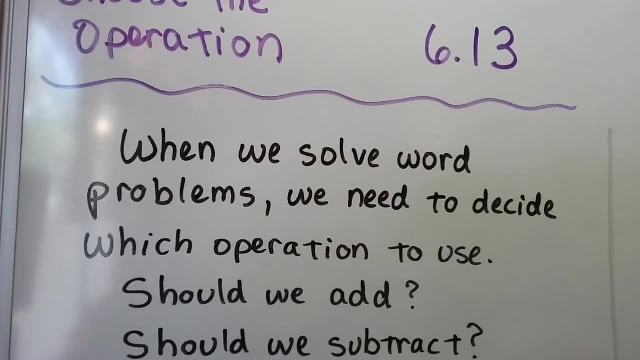 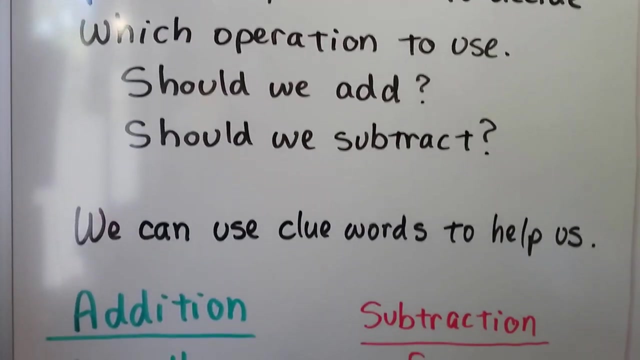 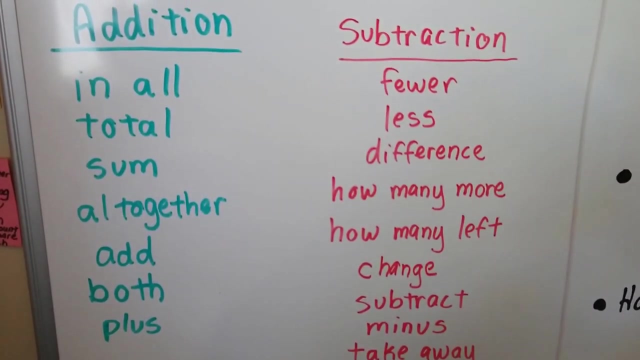 Word problem solving. Choose the operation. Lesson 6.13.. When we solve problems, we need to decide which operation to use. Should we add, Should we subtract? We can use clue words to help us. There's a lot of them. Here's some of them. For addition, you'll see clue words like: in all total sum altogether: 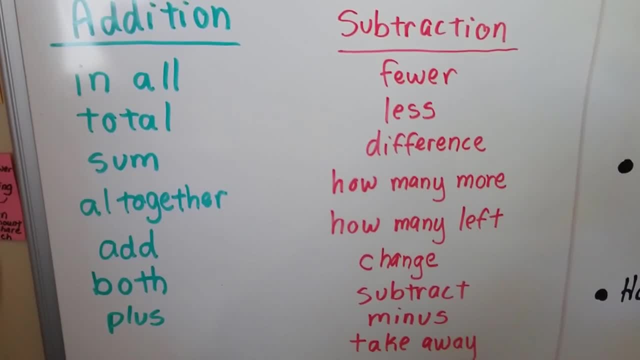 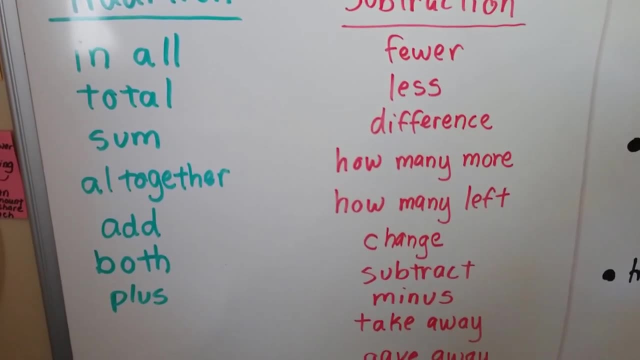 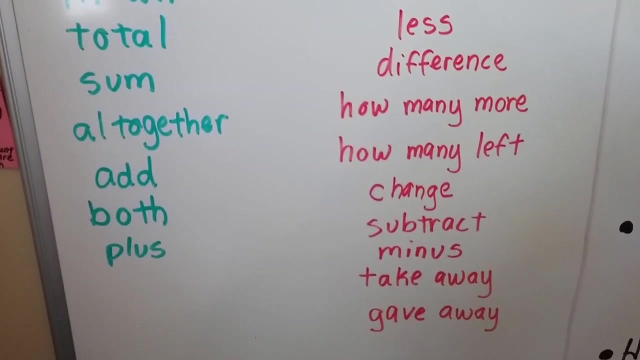 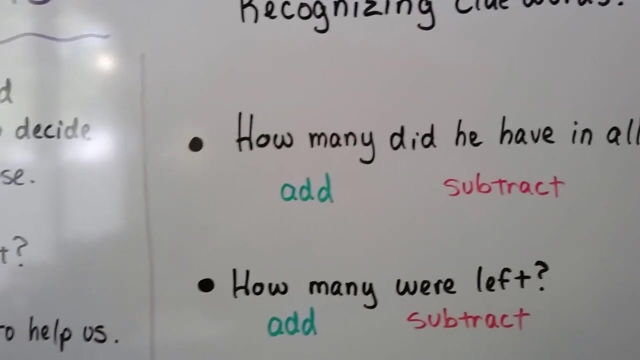 Add both or plus, And in subtraction you'll see words like fewer, less, difference, how many more, how many left, change, subtract, minus, take away or gave away. There's even more than this, but these are the ones that you're going to be dealing with in second grade. It's important that we learn how to recognize clue words. 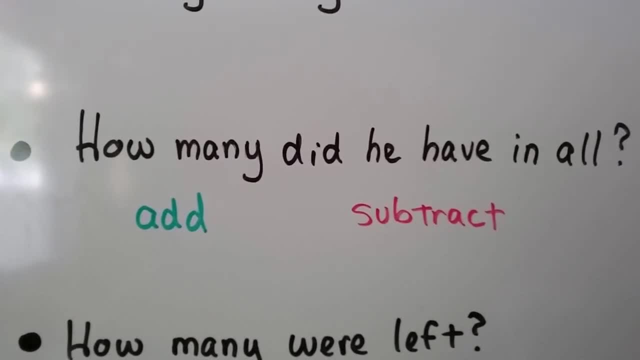 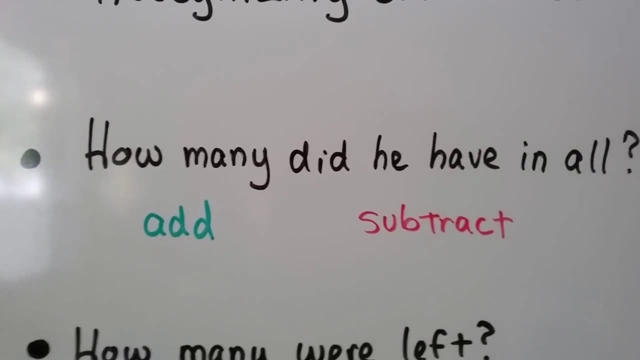 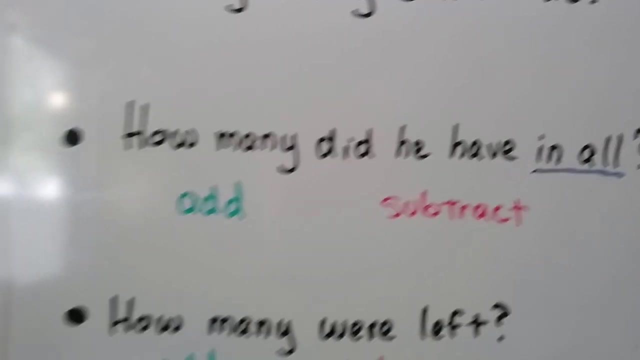 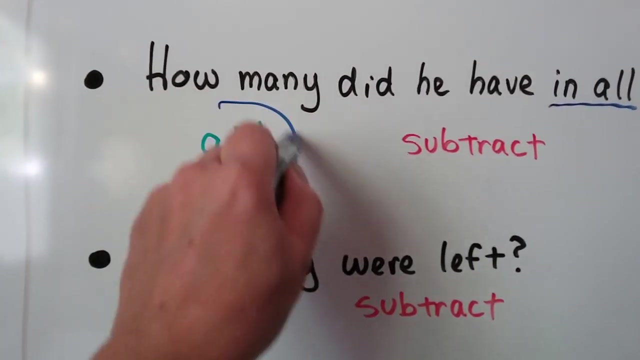 Look at this one. If the word problem said at the end, how many did he have in all, Do you think we would add or subtract? Well, we have to look for the clue words. The clue words here are: in all. We can look on our addition list and see that in all is an addition clue word. So that means we're going to add. You need to find out how many they have in all. 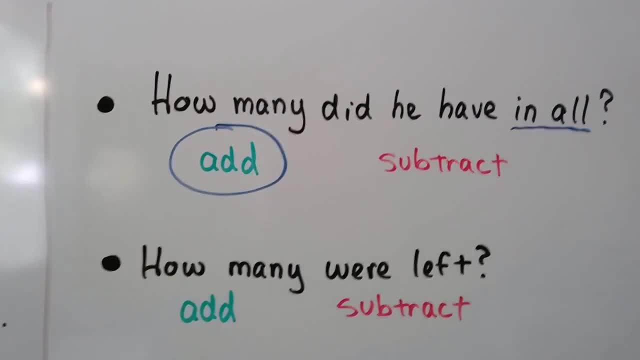 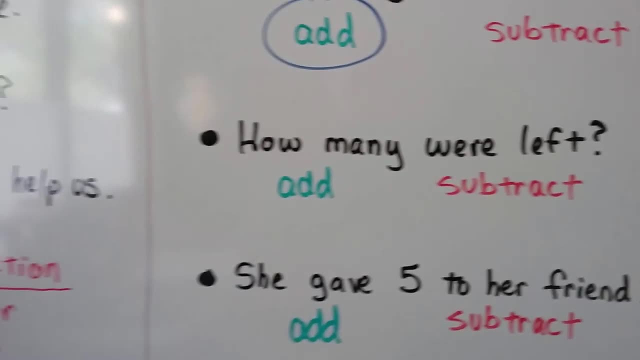 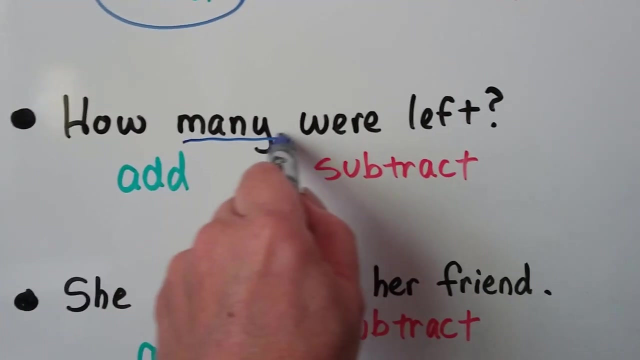 So that means you're going to add two amounts, or three amounts or more. How about this one? How many were left? Well, how many left is a clue word for subtraction. Those are clue words And it tells us that we need to find the difference between two amounts. 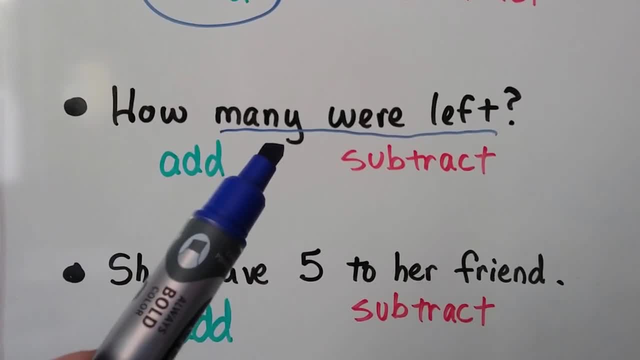 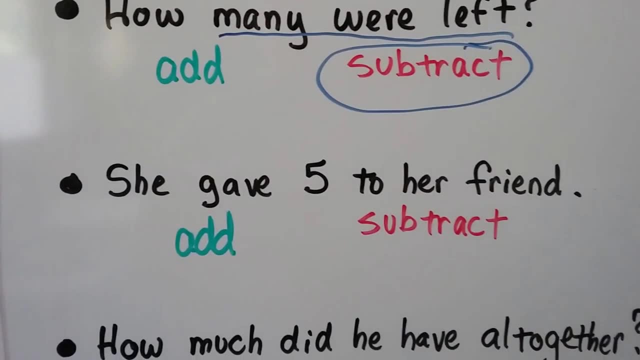 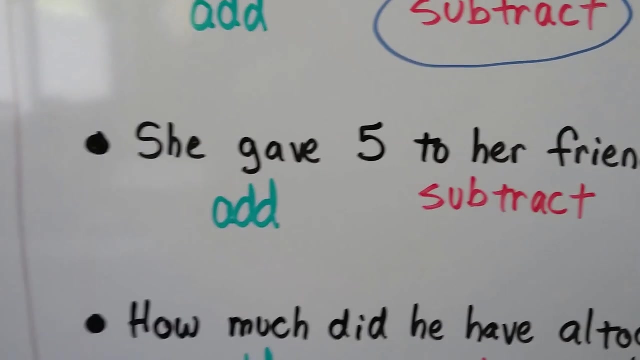 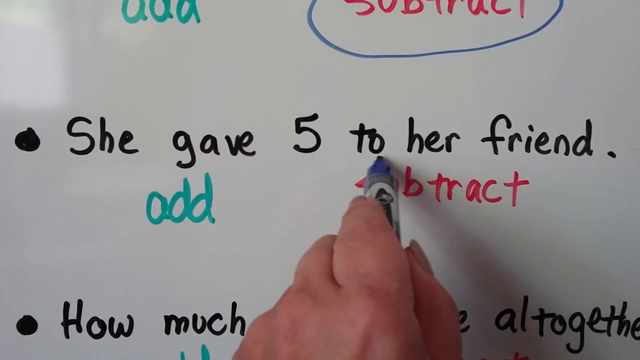 There was an amount. Maybe some were taken away and they want to know how many were left. So that means we're going to subtract to find the difference. She gave five to her friend. So if she gave five to her friend she has less right, And if she has less that means it's subtraction. We need to find what she's got left because she gave some away. 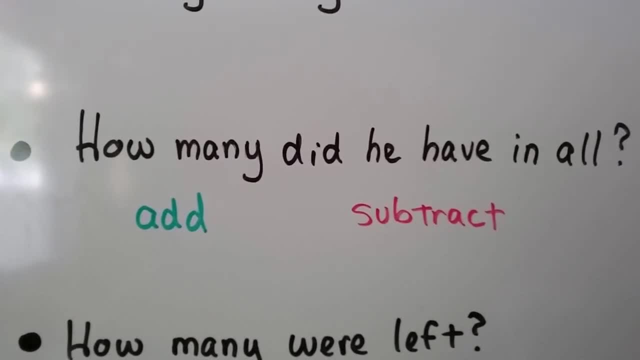 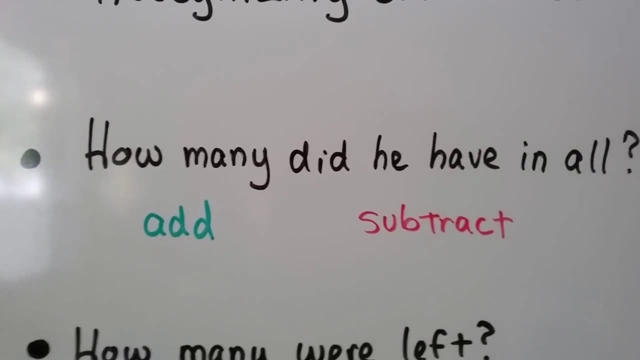 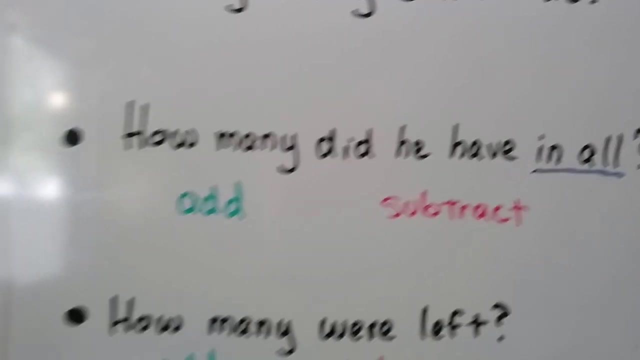 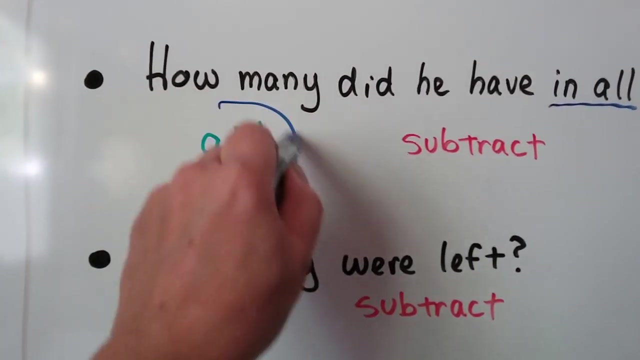 Look at this one. If the word problem said at the end, how many did he have in all, Do you think we would add or subtract? Well, we have to look for the clue words. The clue words here are: in all. We can look on our addition list and see that in all is an addition clue word. So that means we're going to add. You need to find out how many they have in all. 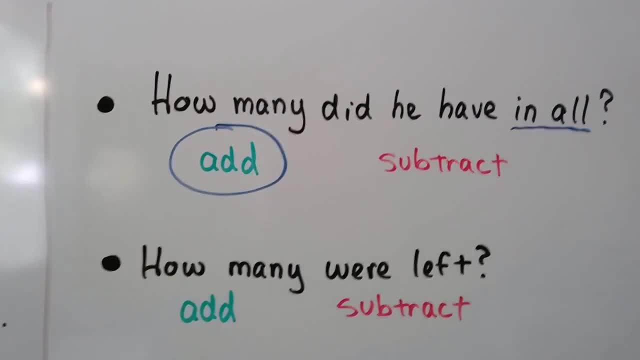 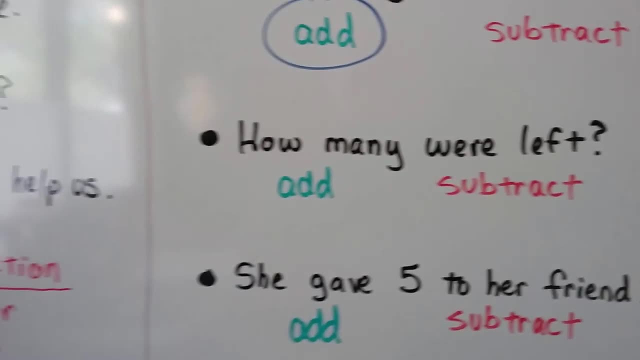 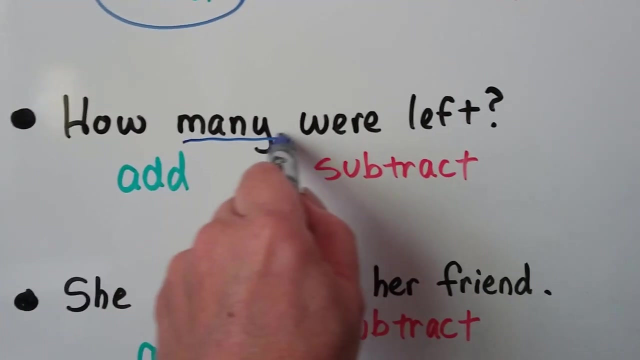 So that means you're going to add two amounts, or three amounts or more. How about this one? How many were left? Well, how many left is a clue word for subtraction. Those are clue words And it tells us that we need to find the difference between two amounts. 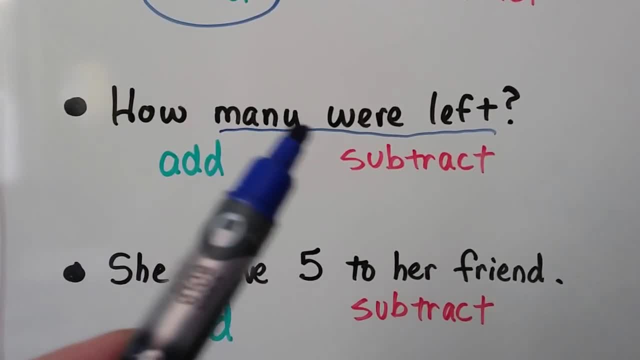 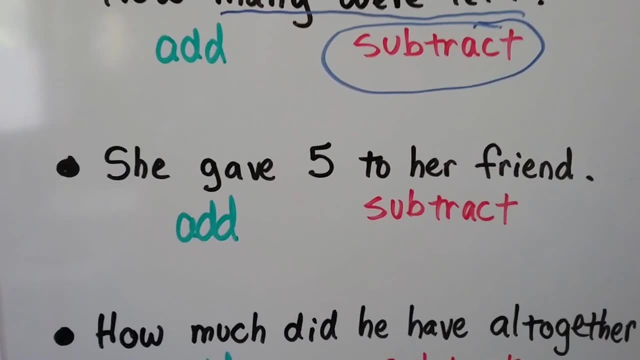 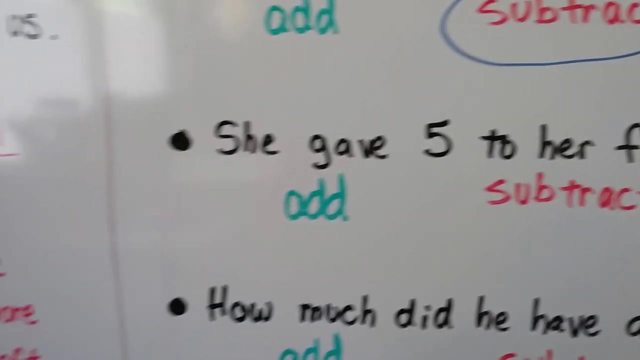 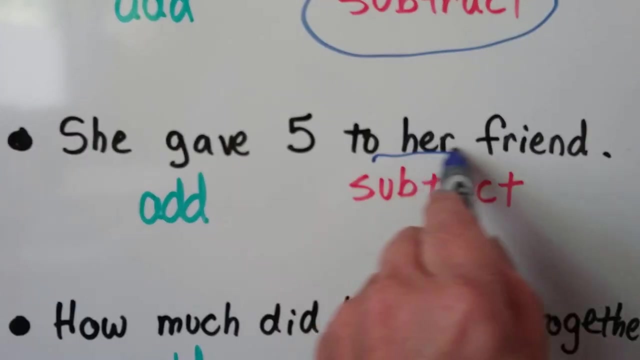 There was an amount. Maybe some were taken away and they want to know how many were left. So that means we're going to subtract to find the difference. She gave five to her friend. So if she gave five to her friend she has less right, And if she has less that means it's subtraction. We need to find what she's got left because she gave some away. 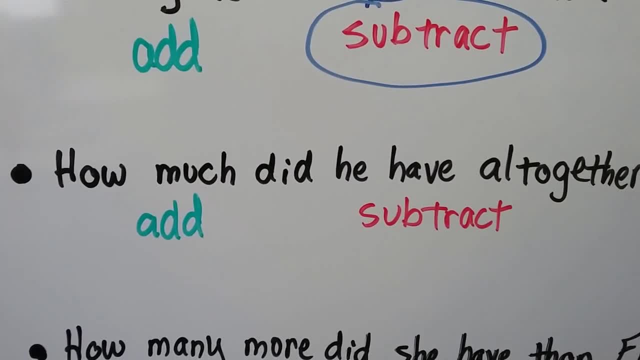 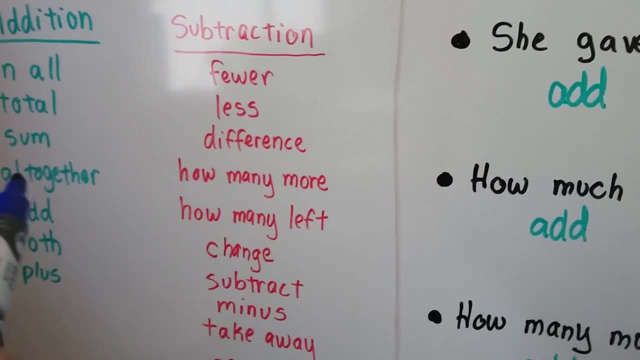 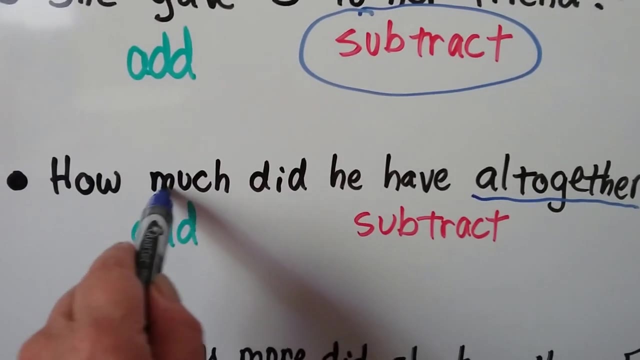 How much did he have altogether? Is that an addition or subtraction operation? If you look at our addition list, altogether is a clue word for addition. This word tells us that we need to add. We're going to find out how much they have altogether. 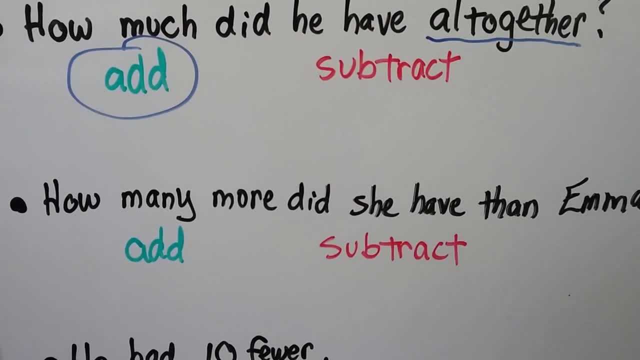 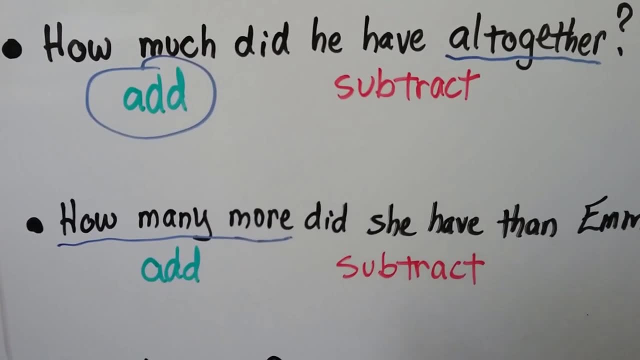 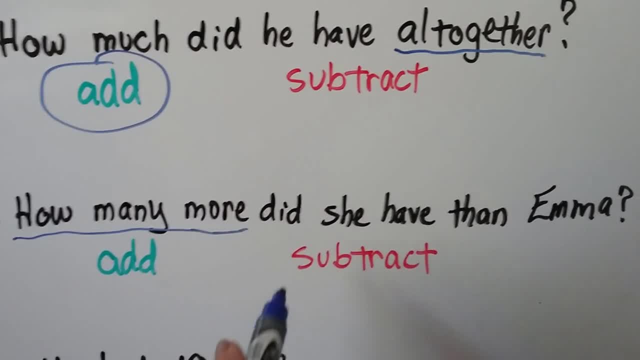 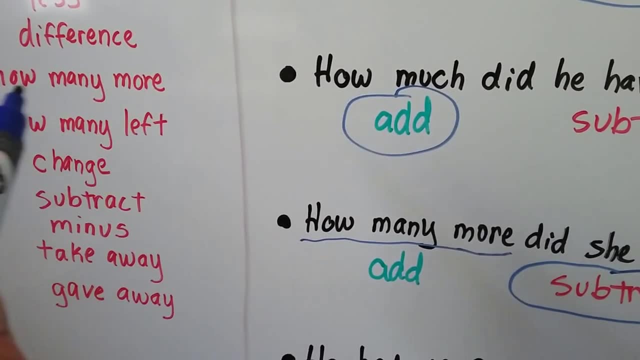 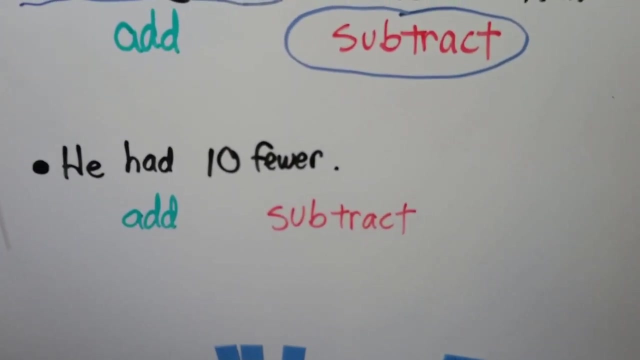 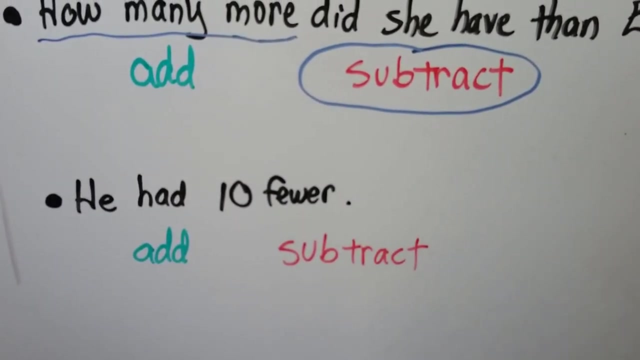 There were two amounts and someone had two, Someone had more than Emma. That means we need to subtract to find the difference in the two amounts. How many more are clue words for subtraction? How about this one? He had ten fewer. If you saw he had ten fewer in a word, problem, do you think you would add or subtract? 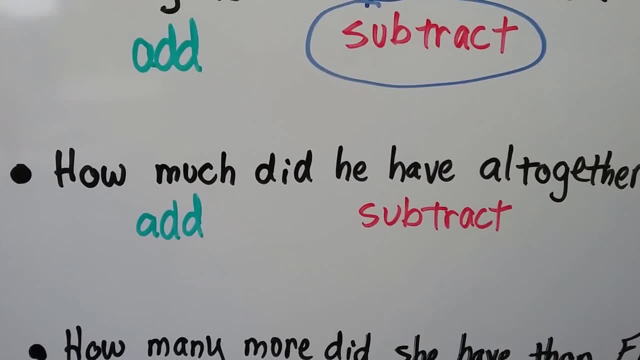 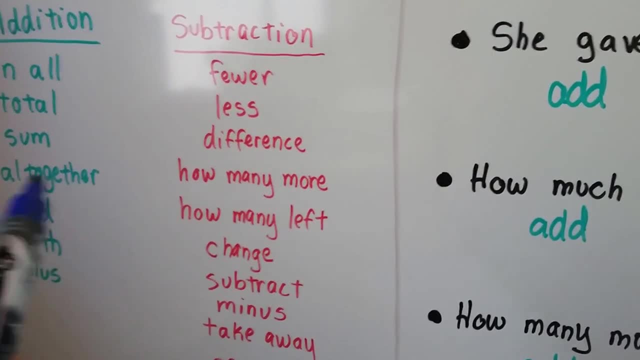 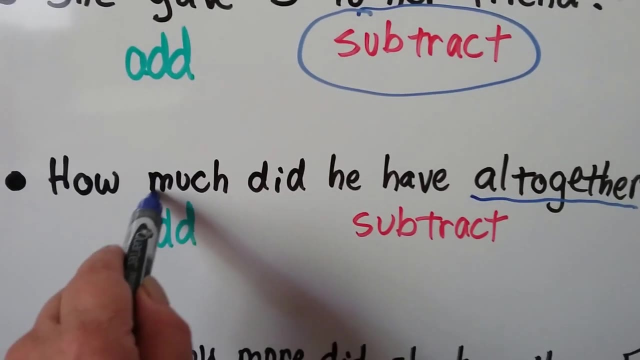 How much did he have altogether? Is that an addition or subtraction operation? If you look at our addition list, altogether is a clue word for addition. This word tells us that we need to add. We're going to find out how much they have altogether. 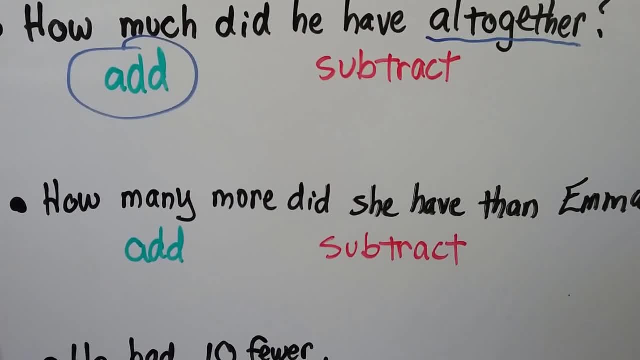 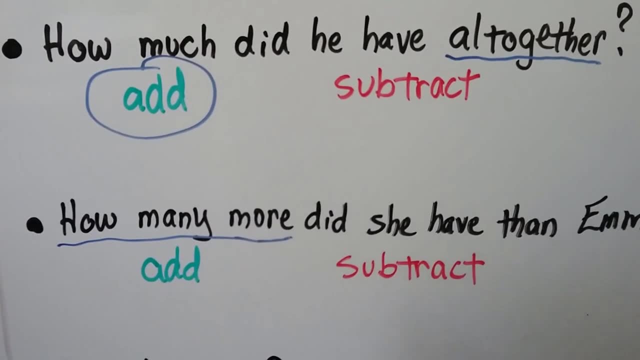 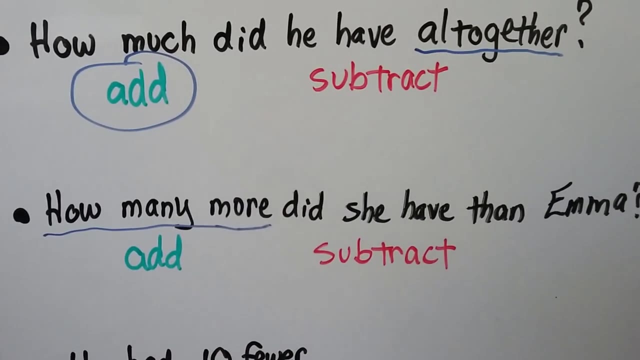 How many more did she have than Emma? Well, how many more? is a clue word that we need to find a difference. There were two amounts and someone had more. Emma had more than Emma. That means we need to subtract to find the difference in the two amounts. 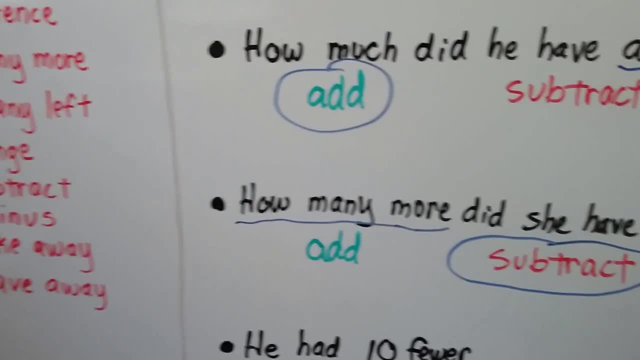 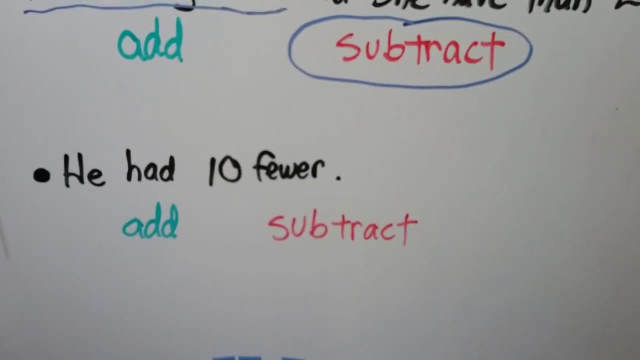 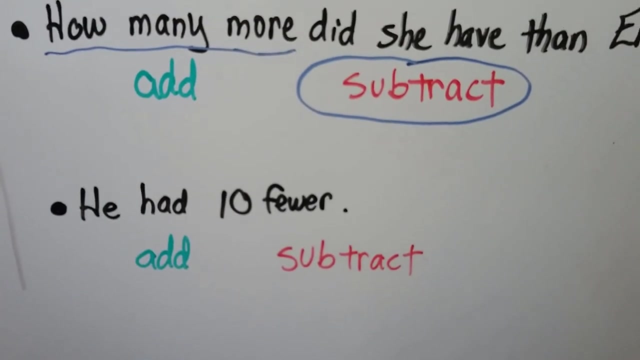 How many more are clue words for subtraction? How about this one? He had ten fewer. If you saw he had ten fewer in a word problem, do you think you would add or subtract? Well, let's look at our clue word list. 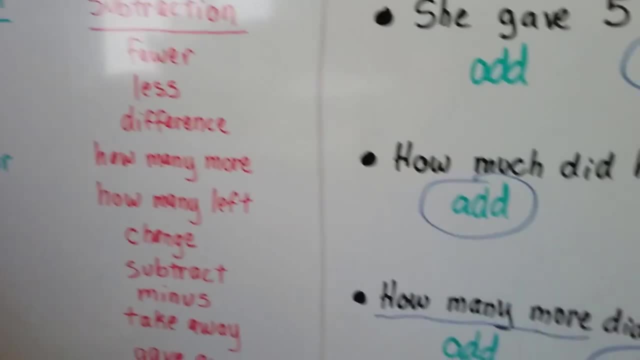 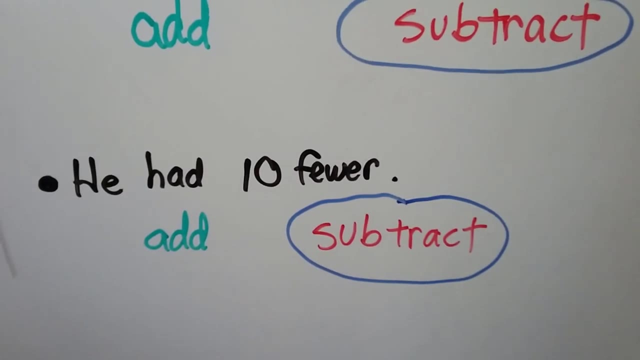 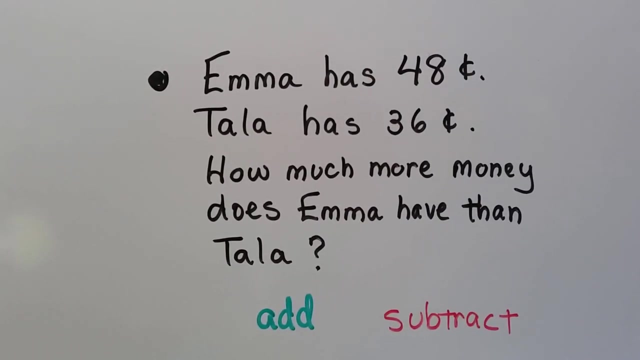 Fewer is a clue word for subtraction, So we would subtract. If he had ten fewer, we would need to take away that ten. We would need to subtract that ten. right? How about this one? Emma has forty-eight cents, Tala has thirty-six cents. 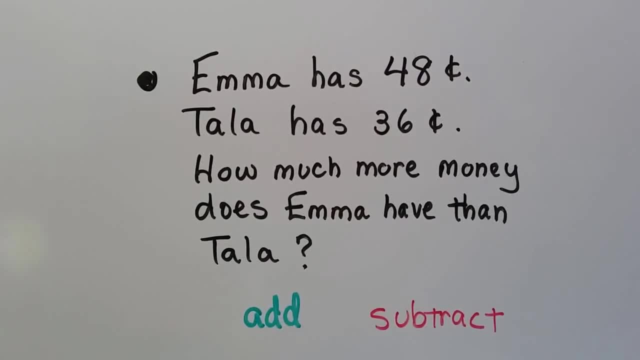 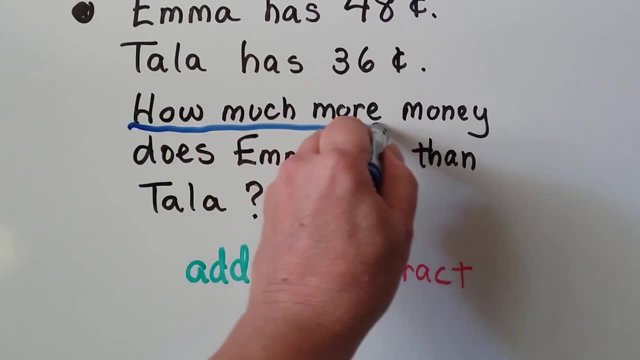 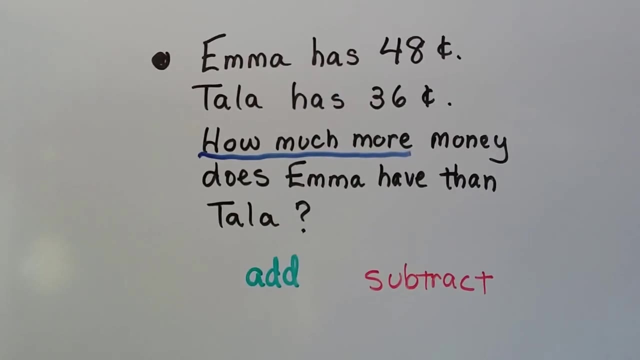 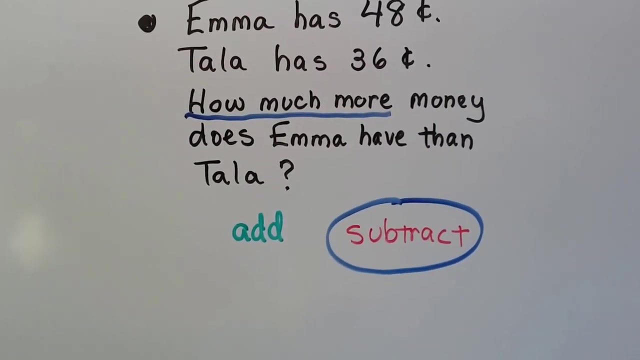 How much more money does Emma have than Tala? You see the clue word right here: How much more. that means we need to find a difference between this amount and that amount, and when we have to find a difference, that's the answer in subtraction. so we need to subtract: how much more? how about? 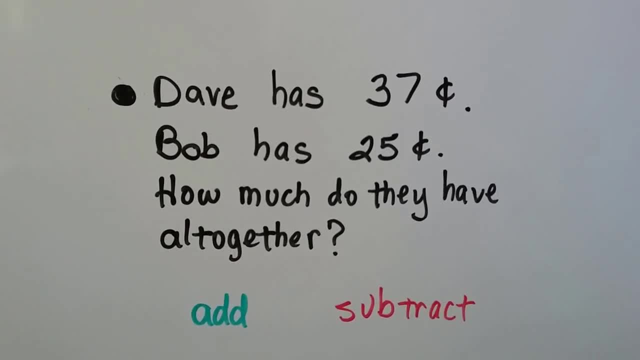 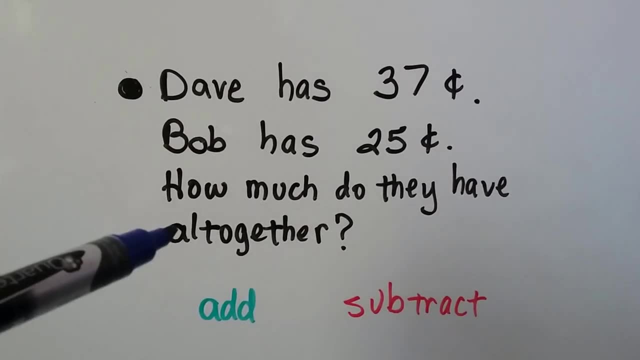 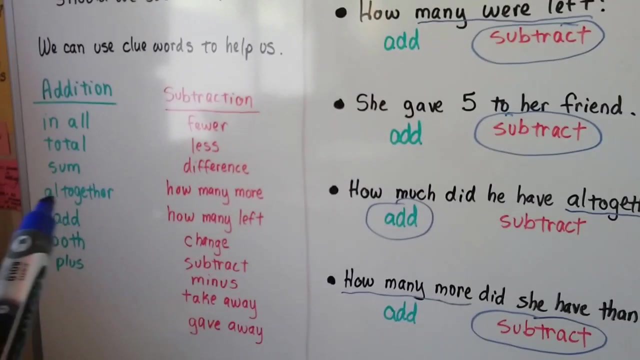 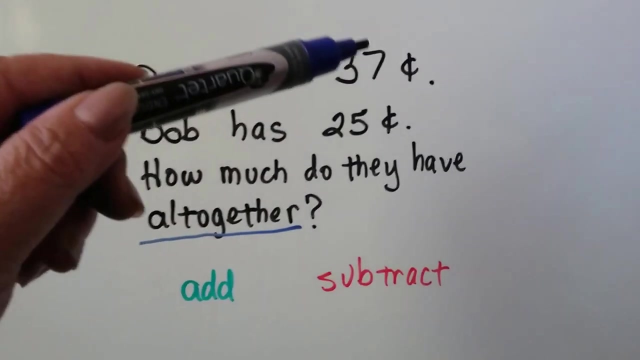 this one. Dave has 37 cents and Bob has 25 cents. how much do they have all together? our clue word here is all together, and if you look at our clue word list, the word all together is in the addition list, isn't it? so we would need to add the 37 cents and the 25 cents. 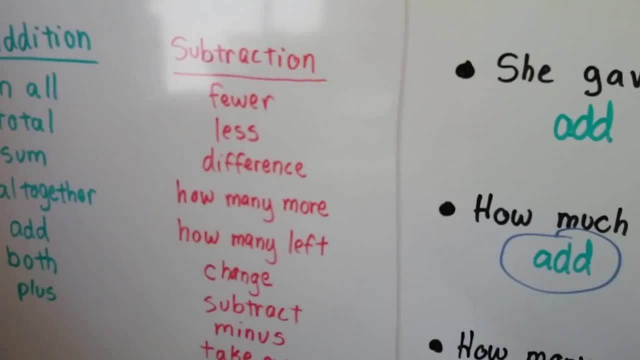 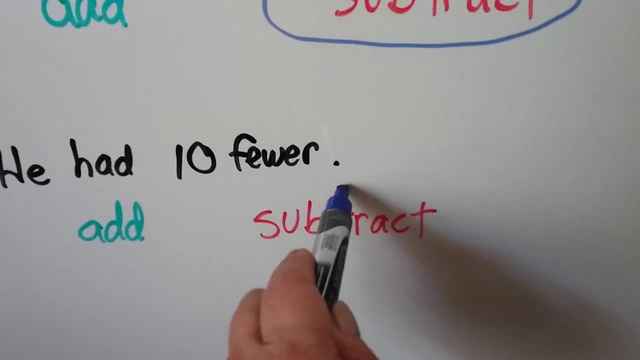 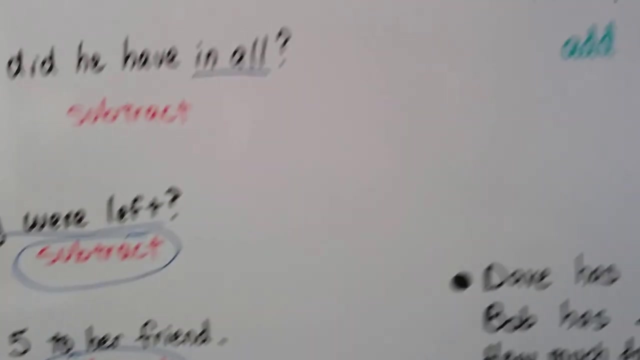 Well, let's look at our clue word list. Fewer is a clue word for subtraction, So we would subtract. If he had ten fewer, we would need to take away that ten. We would need to subtract that ten, right? How about this one? 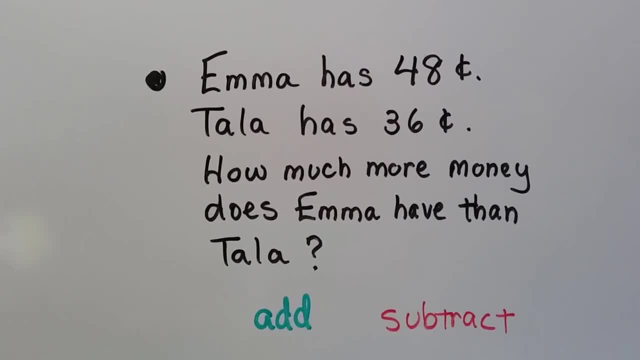 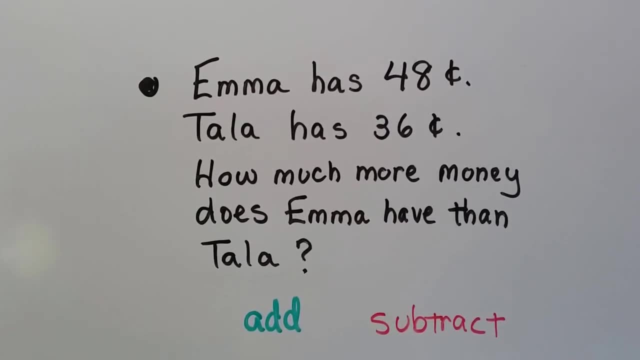 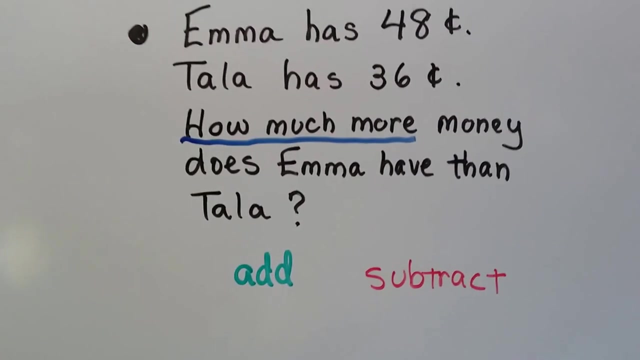 Emma has forty-eight cents. Tala has thirty-six cents. How much more money does Emma have than Tala? You see the clue word right here: How much more. That means we need to find a difference between this amount and that amount. 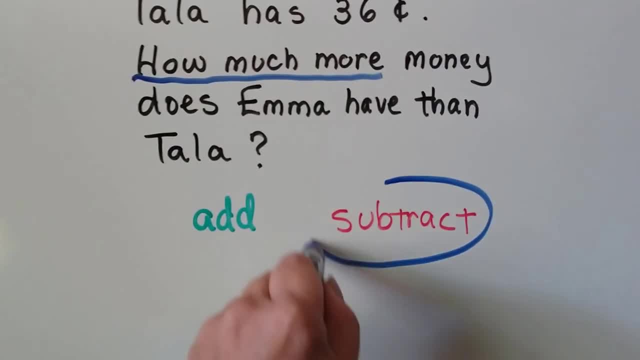 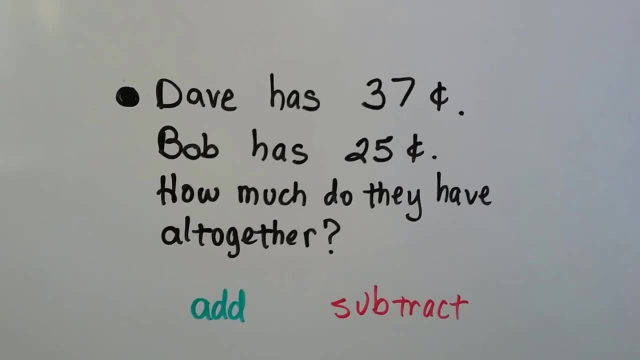 And when we have to find a difference, that's the answer in subtraction. So we need to subtract: How much more? How about this one? Dave has thirty-seven cents and Bob has twenty-five cents. How much do they have altogether? How much do they have altogether? 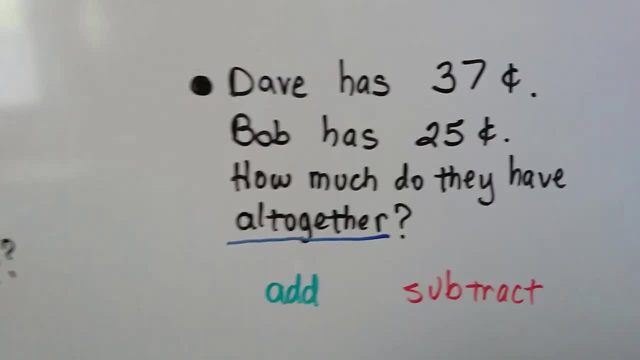 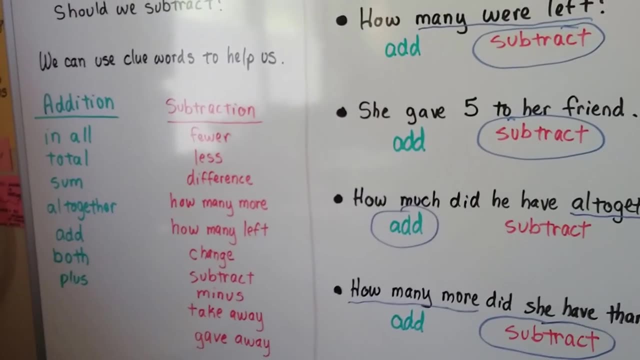 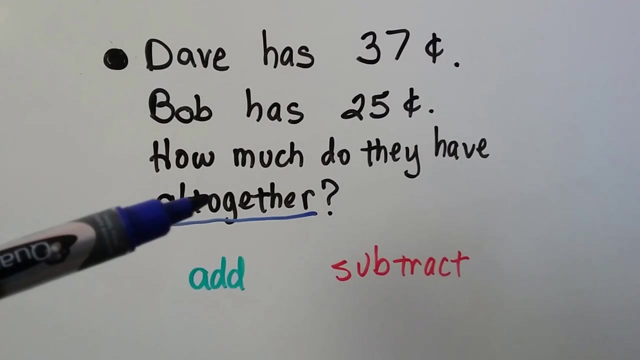 Our clue word here is altogether, And if you look at our clue word list, the word altogether is in the addition list, isn't it? So we would need to add the thirty-seven cents and the twenty-five cents altogether to find out how much they had in all, wouldn't we? 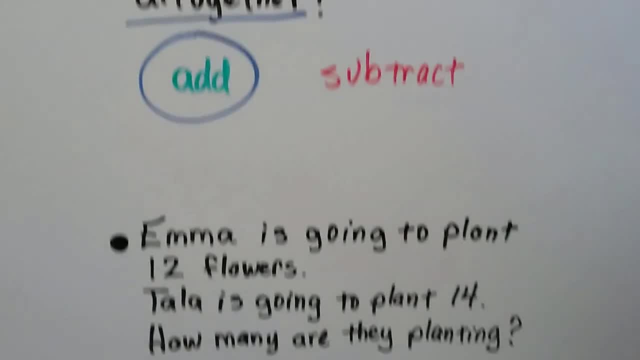 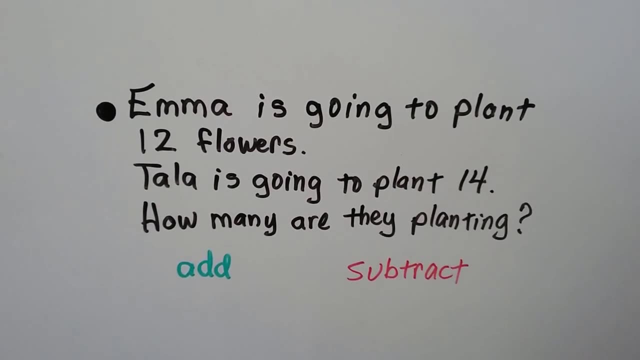 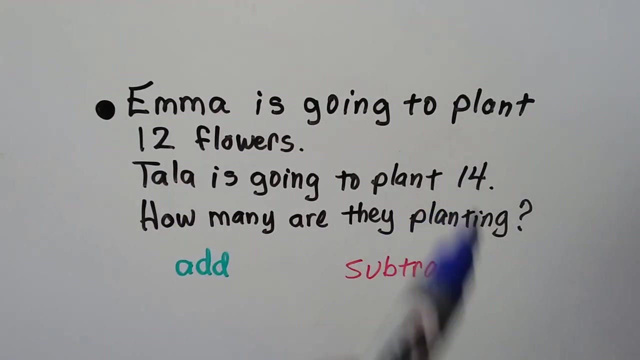 So we would add: Okay, how about this one? Emma is going to plant twelve flowers, Tala is going to plant fourteen. How many are they planting? Well, it's important that Emma is planting twelve and Tala is planting fourteen. 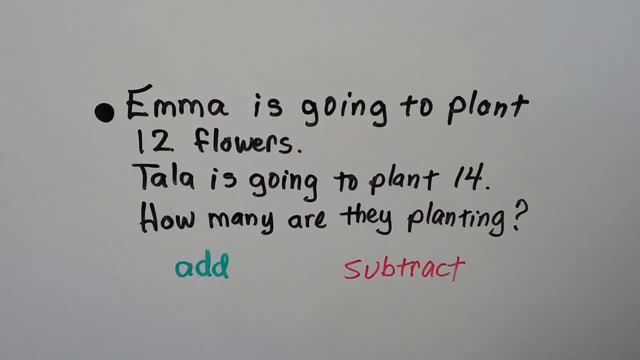 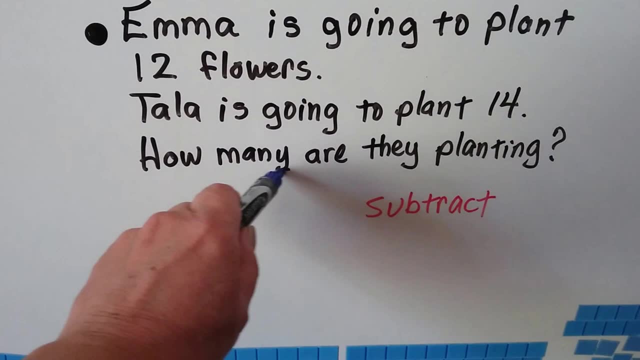 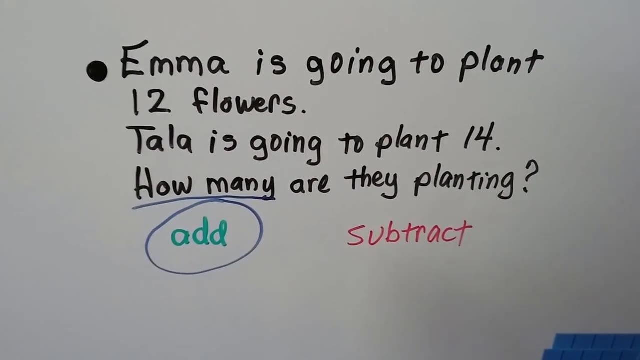 but is this adding or subtracting? It doesn't ask how many more Tala is planting than Emma. It says how many are they planting. So how many is telling us to add? We need to add Emma's and Tala's together to find out how much they're planting in all. 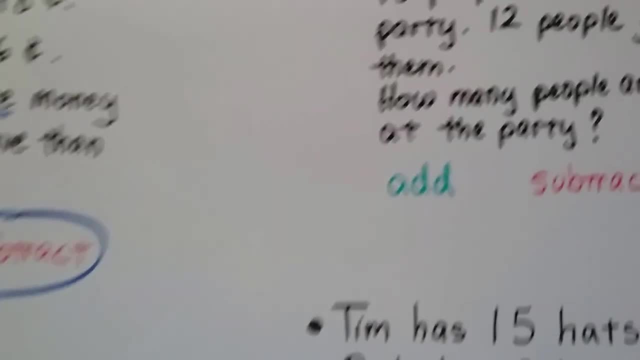 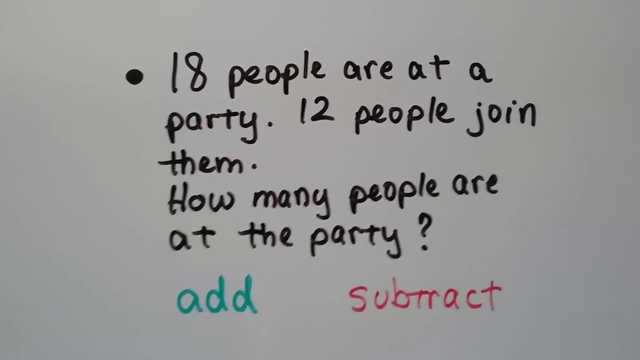 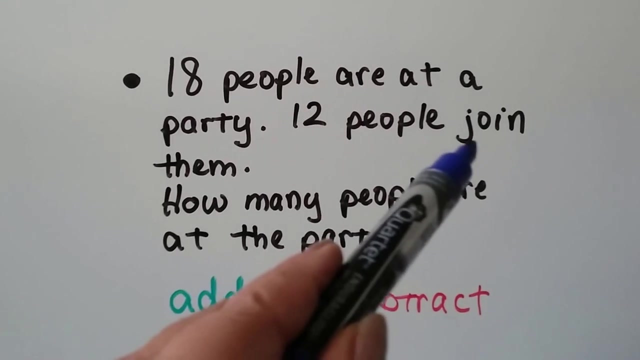 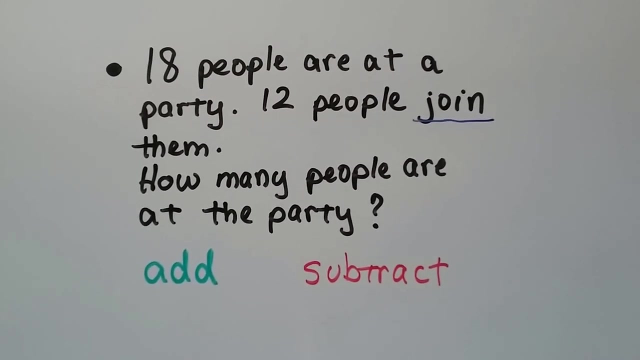 So that's addition. Okay, we've got another one. Eighteen people are at a party. Twelve people join them. How many people are at the party? Would we add or subtract? See the word join. This word join tells us that we're combining, we're putting the numbers together, we're joining them. 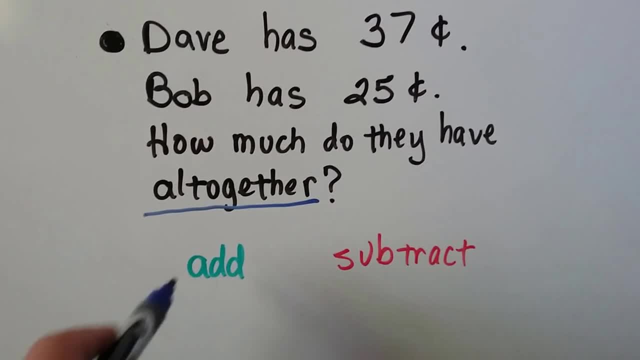 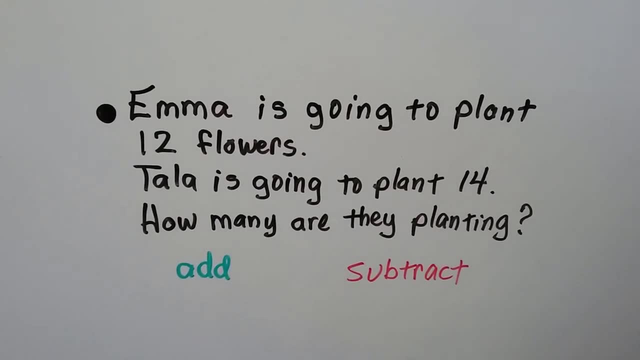 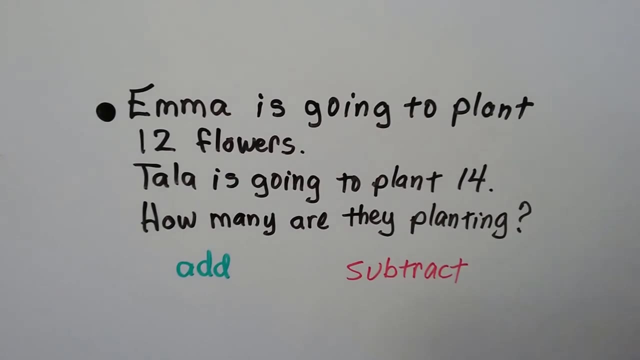 all together to find out how much they had in all, wouldn't we? so we would add: okay, how about this one? Emma is going to plant 12 flowers. 12 flowers. Tala is going to plant 14. how many are they planting? well, it's important that Emma's planting 12 and Tala's planting 14, but is this adding or? 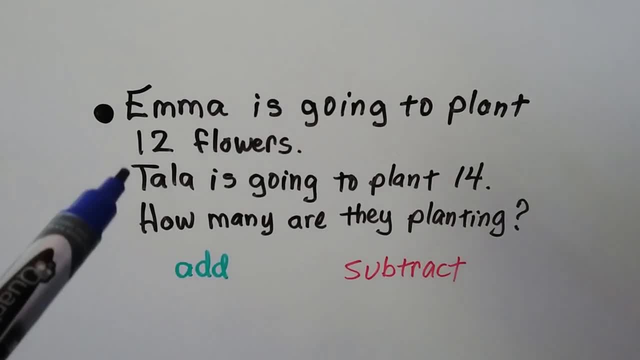 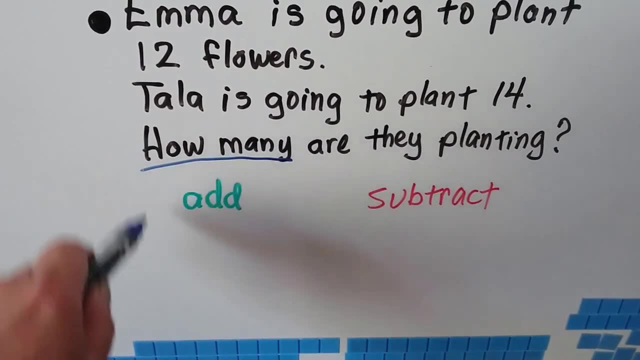 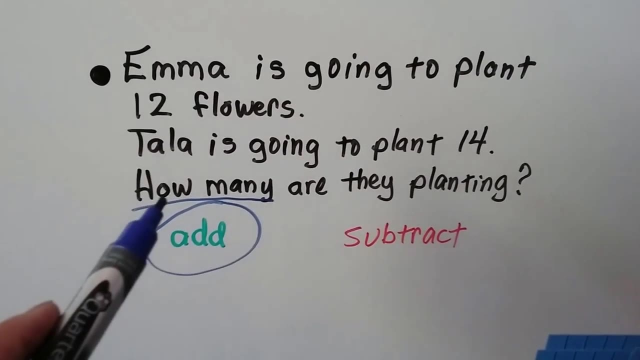 subtracting. it doesn't ask how many more Tala's planting than Emma. it says how many are they planting, so how many is telling us to add? we need to add Emma's and Tala's together to find out how much they're planting in all. 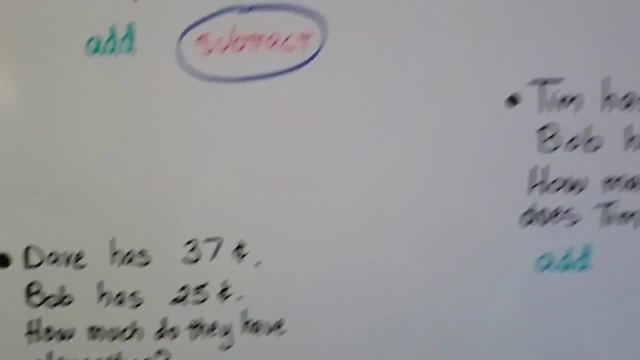 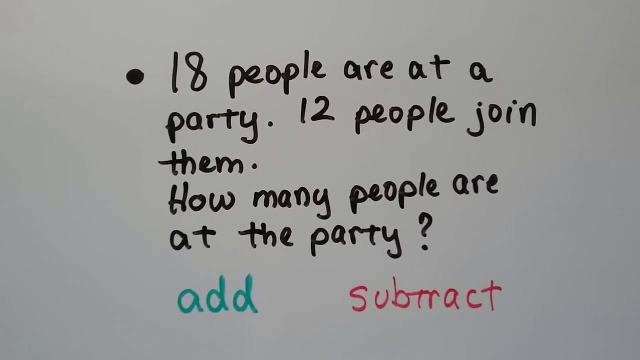 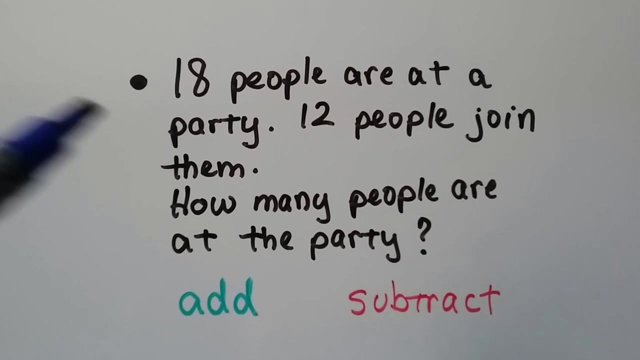 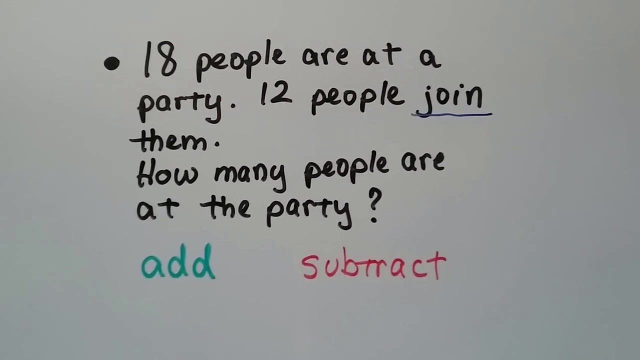 that's Additionught at how many people are at the party. would we add or subtract? seeing the word join? this is where Join tells us that we're combining. we're putting the numbers together, we're joining them. that means we're gonna add them. and we're putting the numbers together, we're joining them, so it means we're gonna add them. 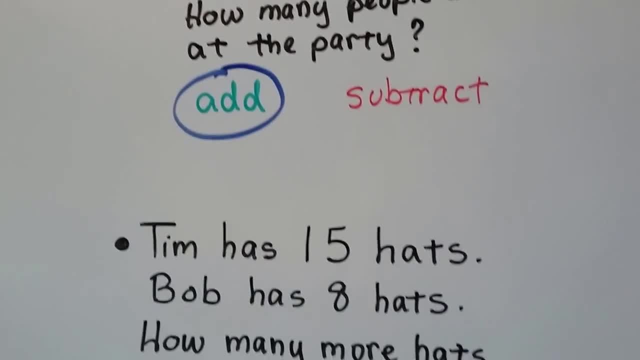 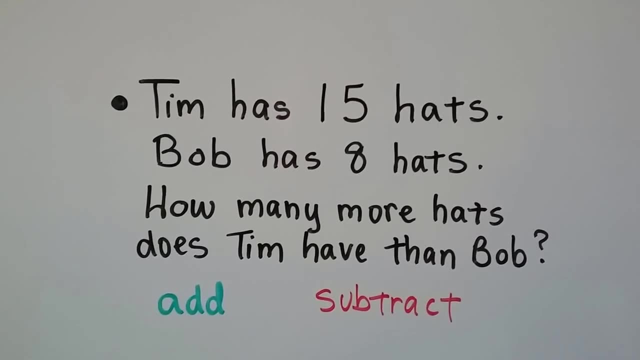 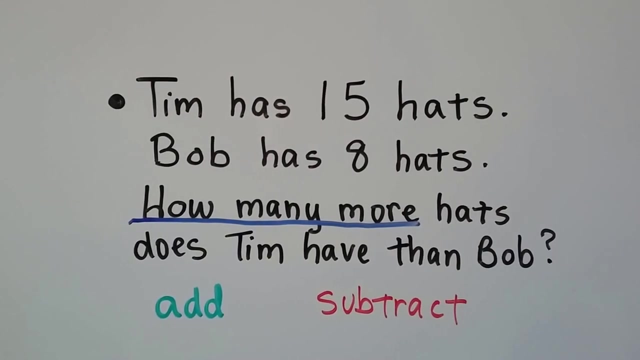 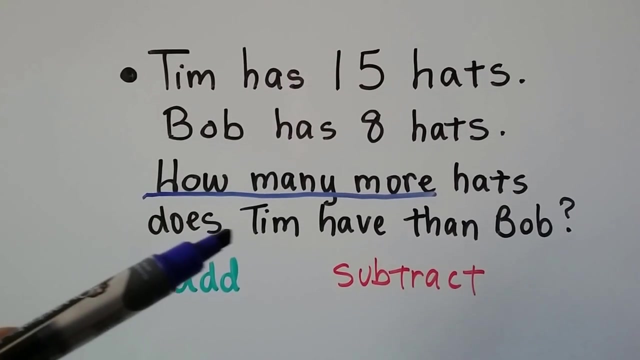 this means we're gonna add them. Tim has 15 hats. Bob has 8 hats. How many more hats does Tim have than Bob? How many more is the clue word for subtraction. We need to compare and find the difference between 15 and 8.. And that would be how many more Tim would have than Bob. So that tells. 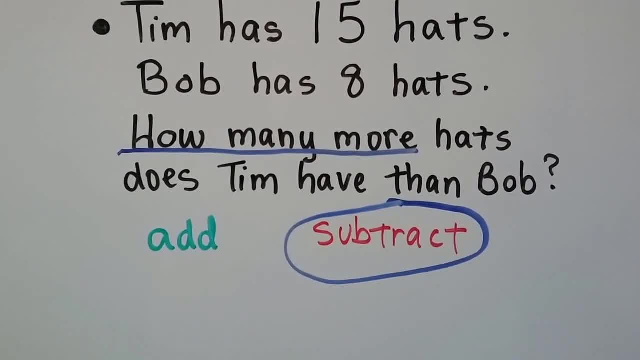 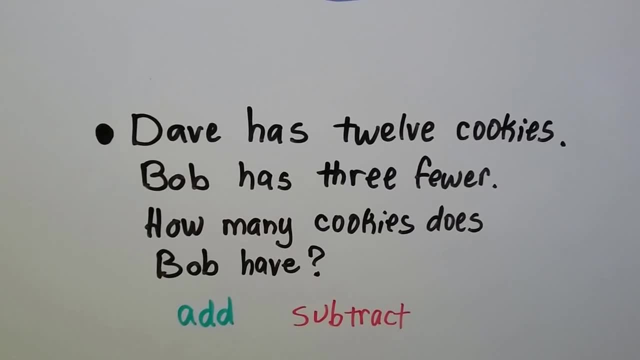 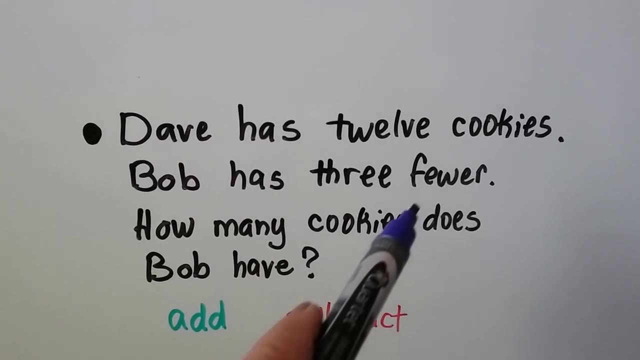 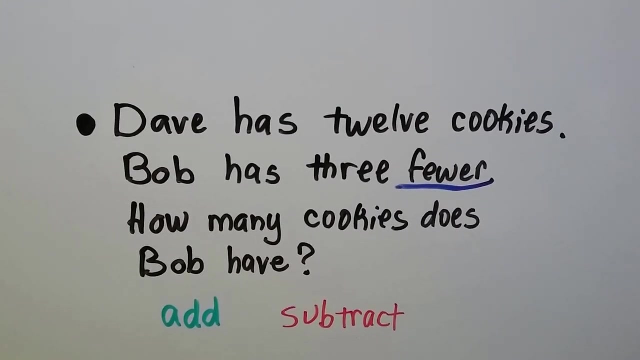 us subtraction. How many more is clue words for subtraction. Dave has 12 cookies. Bob has 3 fewer. How many cookies does Bob have? See the word fewer. Fewer is a clue word. Do you know if it's for addition or subtraction? If you said subtraction, you're right. 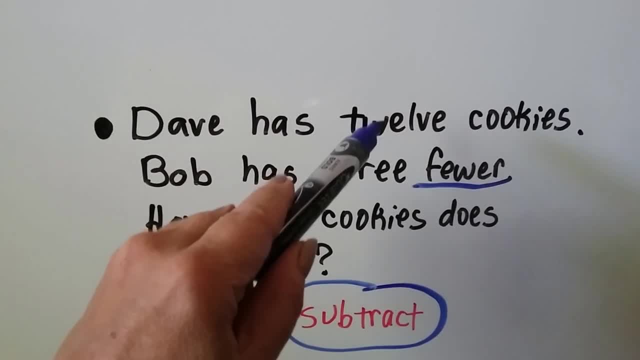 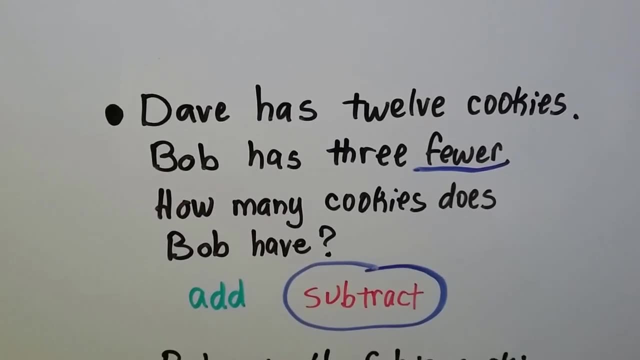 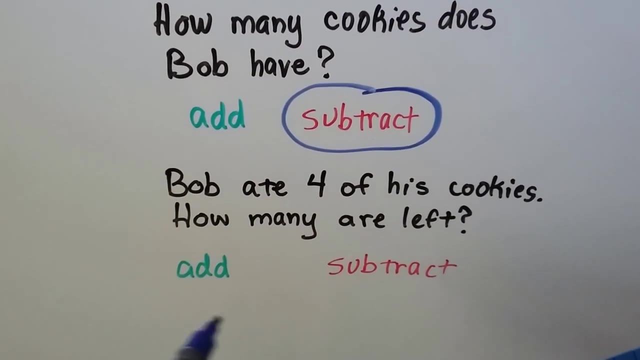 We would subtract 3 from 12. And that would tell us how many Bob has, Because he has 3 fewer, 3 less than 12.. Bob ate 4 of his cookies. How many are left? Is that addition or subtraction? 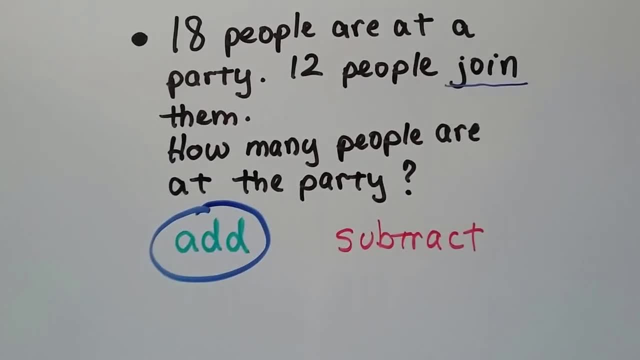 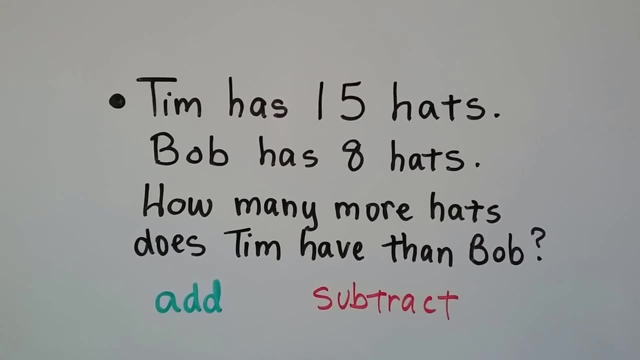 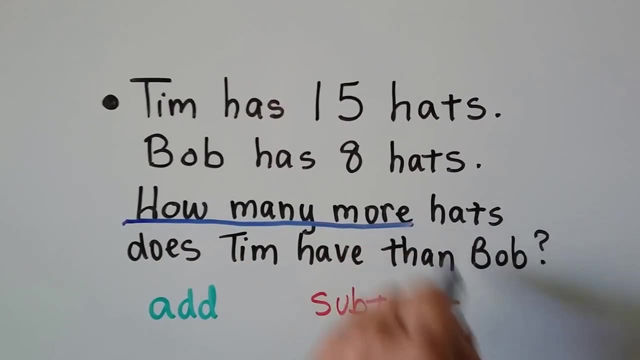 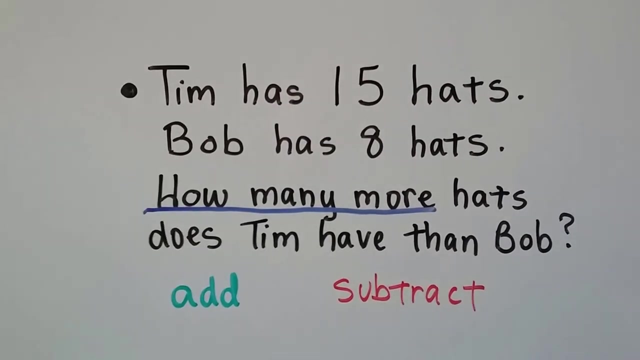 So that means we're going to add them. Okay, Tim has fifteen hats. Bob has eight hats. How many more hats does Tim have than Bob? How many more is? clue word for subtraction. We need to compare and find the difference between fifteen and eight. 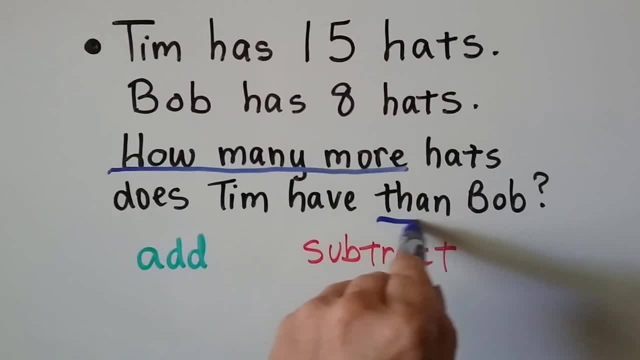 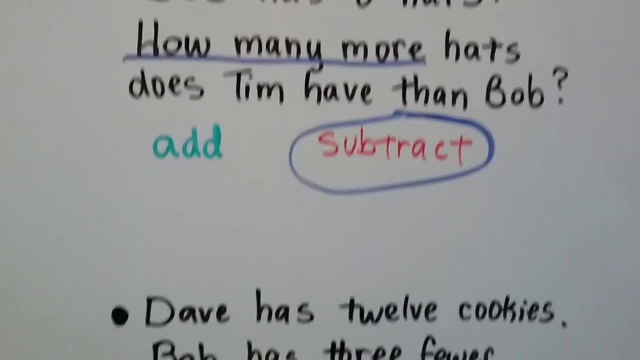 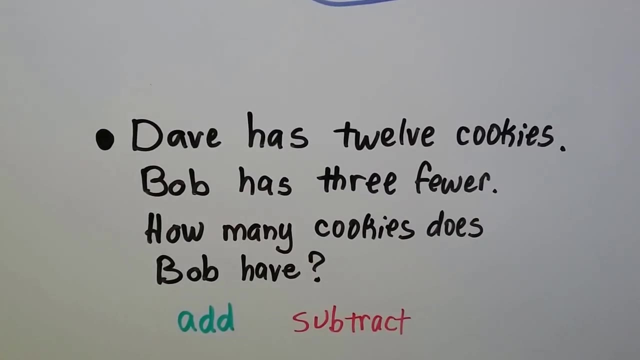 And that would be how many more Tim would have than Bob. So that tells us: subtraction, Subtraction. How many more is clue words for subtraction? Dave has twelve cookies, Bob has three fewer. How many cookies does Bob have? See the word fewer. 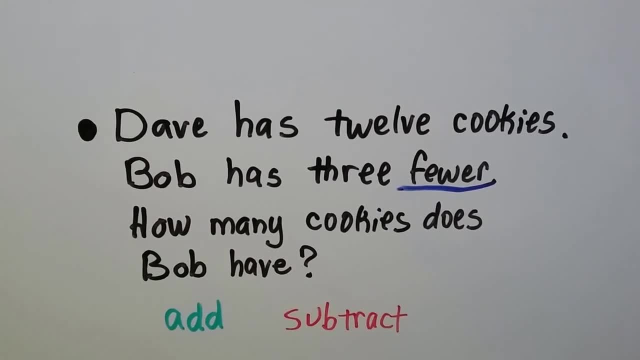 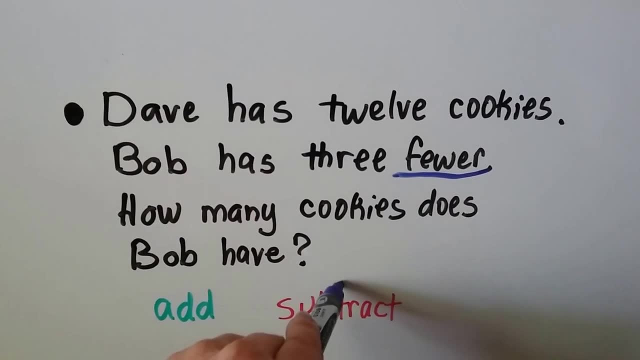 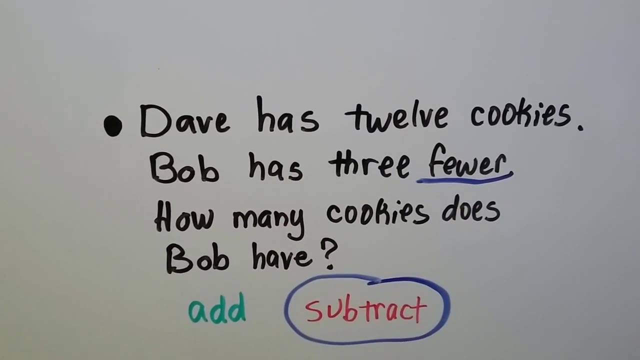 Fewer is a clue word. Do you know if it's for addition or subtraction? If you said subtraction, you're right. We would subtract three from subtraction, Subtraction Three from twelve, And that would tell us how many Bob has. 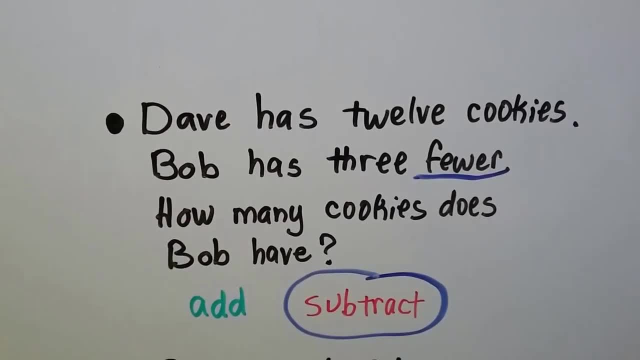 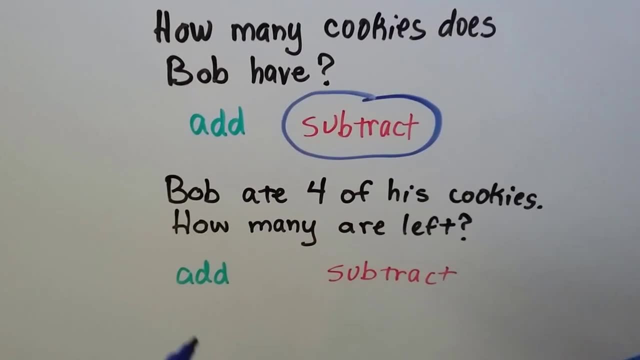 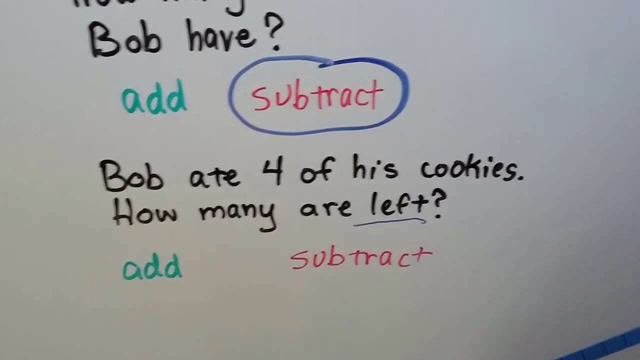 Because he has three fewer, Three less than twelve. Bob ate four of his cookies. How many are left? Is that addition or subtraction? Well, it's asking how many are left, And that's a clue word for subtraction. He ate four, so we take four away. 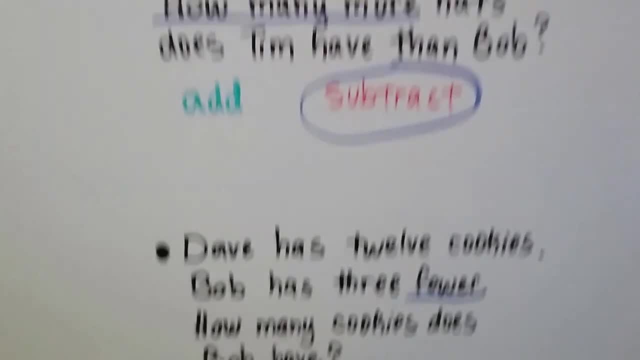 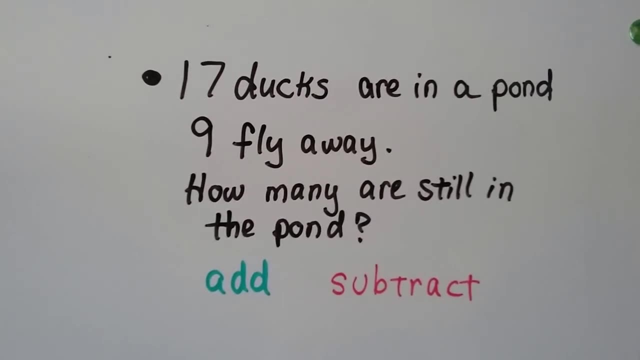 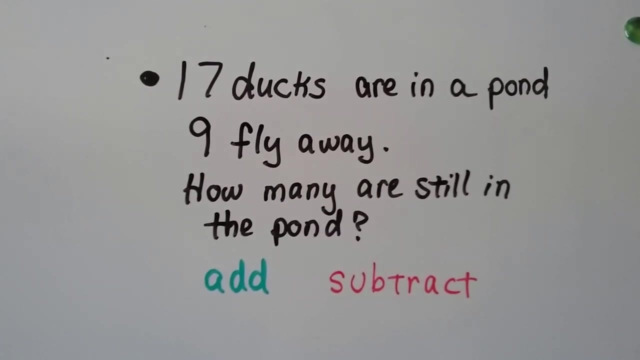 That's subtraction. We got a couple more. There are seventeen ducks in a pond. Nine fly away. How many are still in the pond? Is that add or subtract? Do you know? Do you see any clue words? Well, it says that nine fly away. 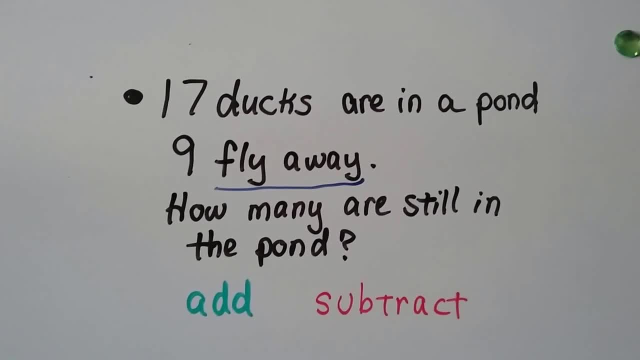 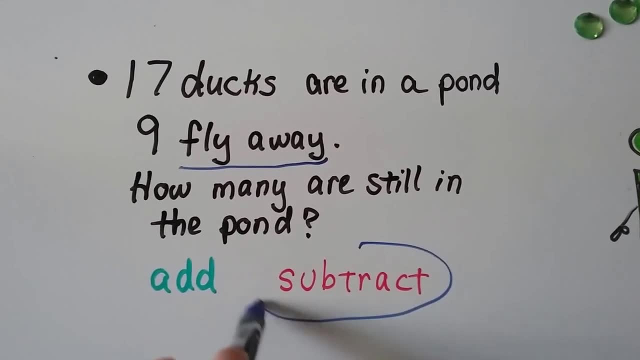 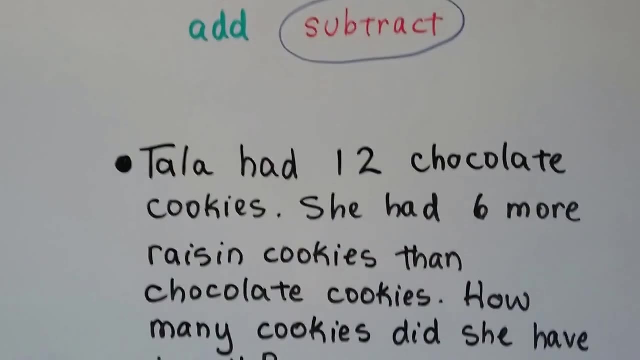 That means they left, They're gone. So we need to find out what seventeen minus nine is. So that's subtraction. That'll tell us how many are still in the pond. We find the difference between the two numbers. Tala had twelve chocolate cookies. 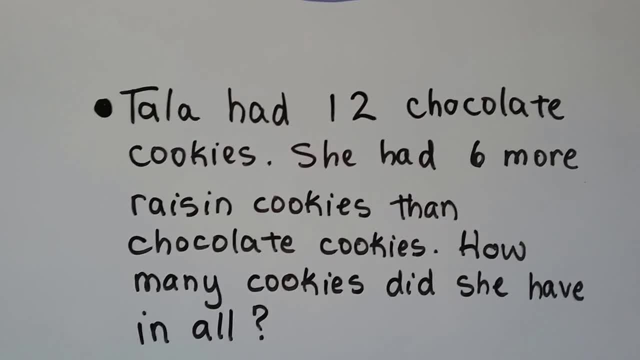 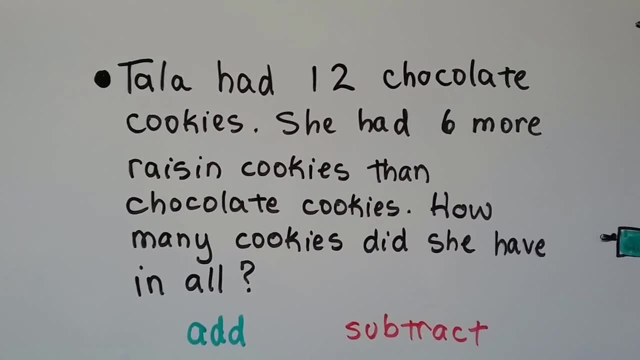 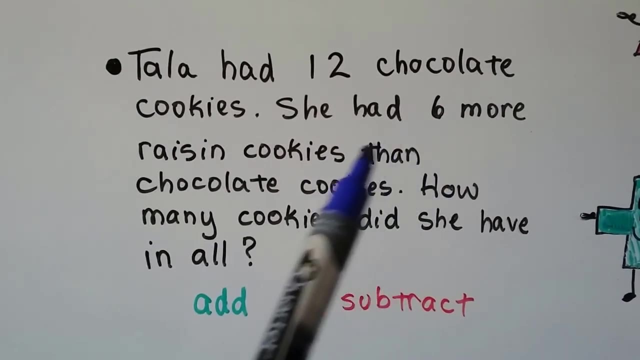 She had six more raisin cookies than chocolate cookies. How many cookies did she have in all? Is this add or subtract? Well, actually there's two parts to this. The first part is we have to find out what six more than twelve is. 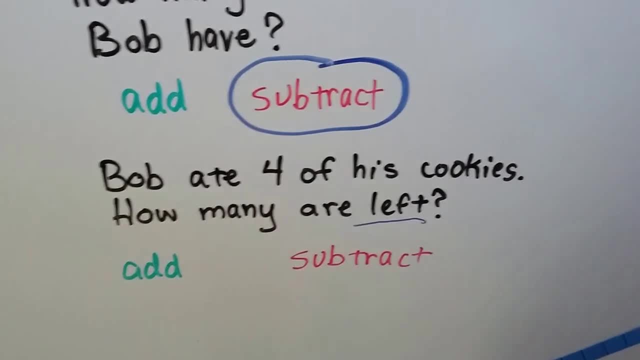 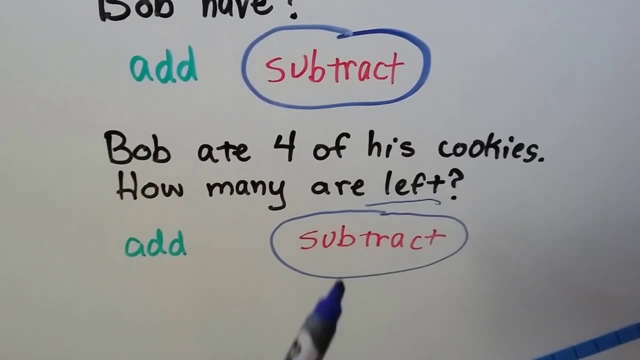 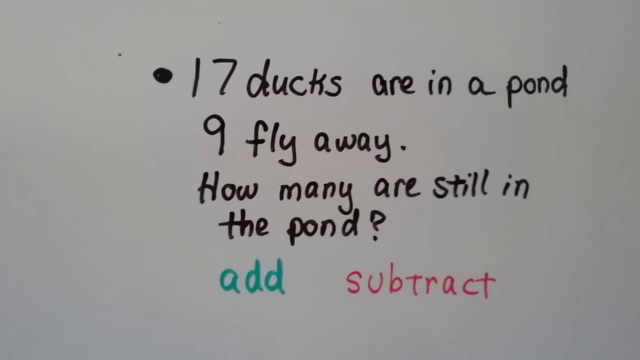 Well, it's asking how many are left, And that's a clue word for subtraction. He ate 4, so we take 4.. Yeah, Or we subtract 4 away. That's subtraction. We have a couple more. There are 17 ducks in a pond. 9 fly away. What's subtract 8?? 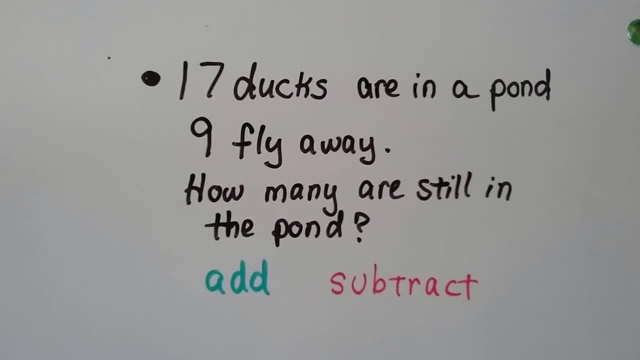 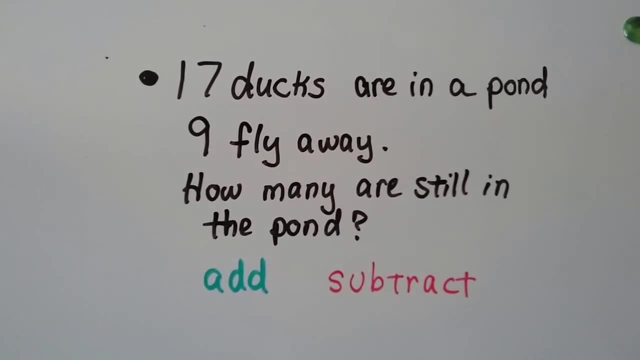 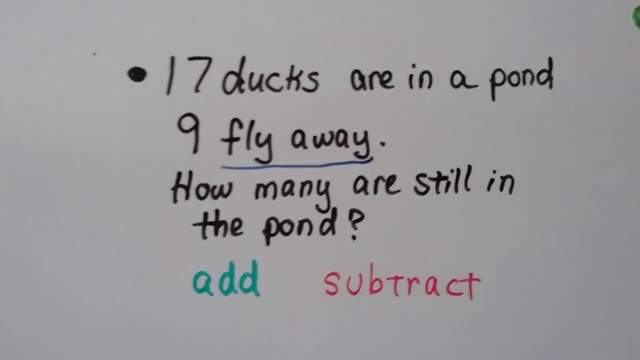 9 fly away. How many are still in the pond? Is that add or subtract? Do you know? Do you see any clue words? Well, it says that 9 fly away. That means that they left. They're gone. So we need to find out how many duck ducks is 15.. 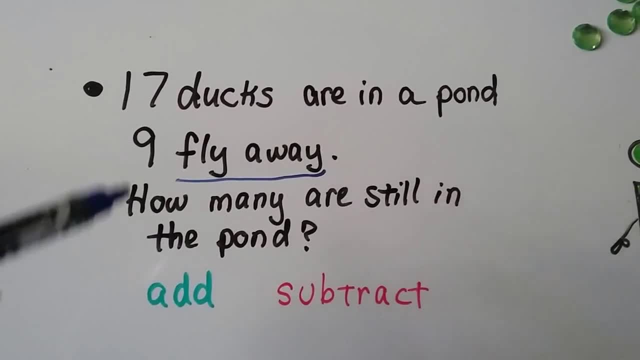 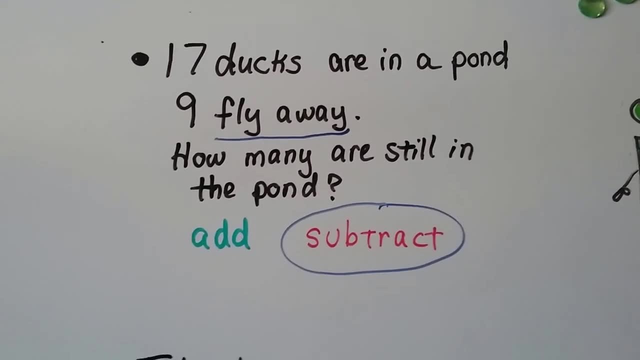 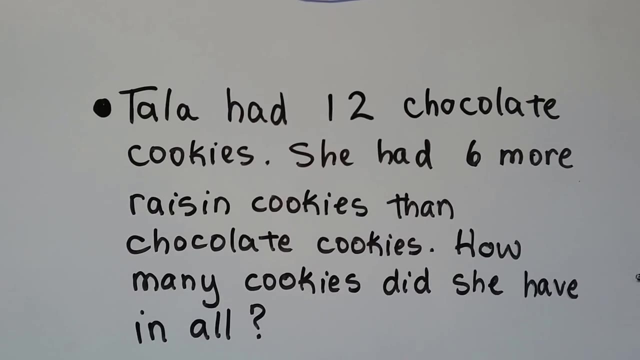 what 17 minus 9 is. So that's subtraction. That'll tell us how many are still in the pond. We find the difference between the two numbers. Tala had 12 chocolate cookies. She had six more raisin cookies than chocolate cookies. How many cookies? 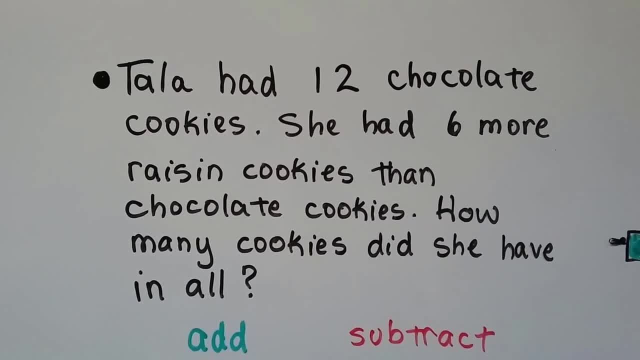 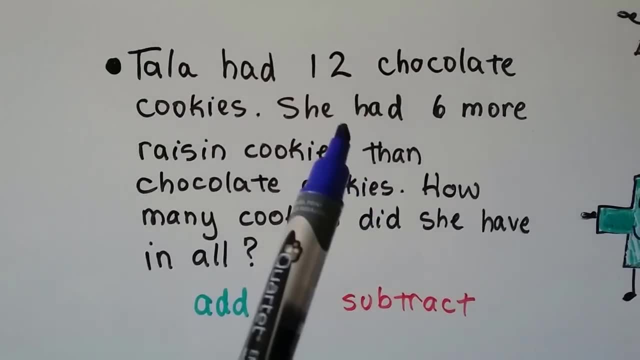 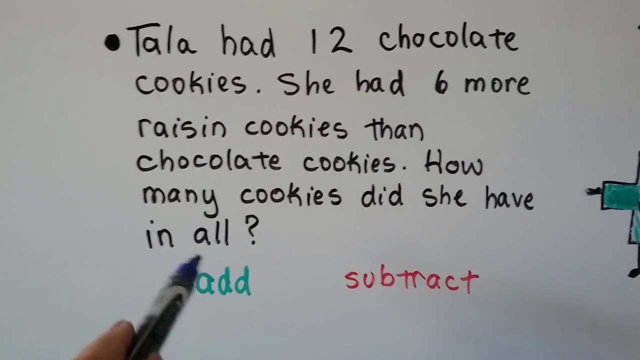 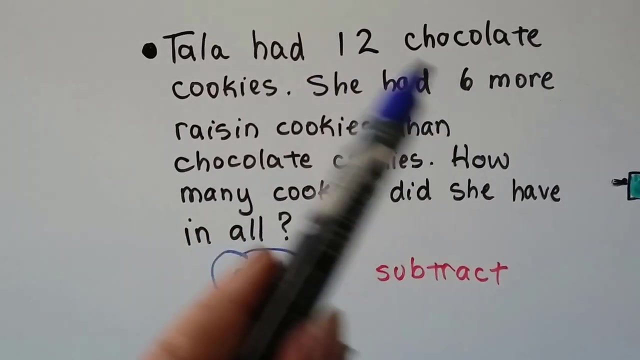 did she have in all? Is this add or subtract? Well, actually there's two parts to this. The first part is we have to find out what 6 more than 12 is. So we have to add 6 plus 12.. So that's adding. Then we have to find what that number is. 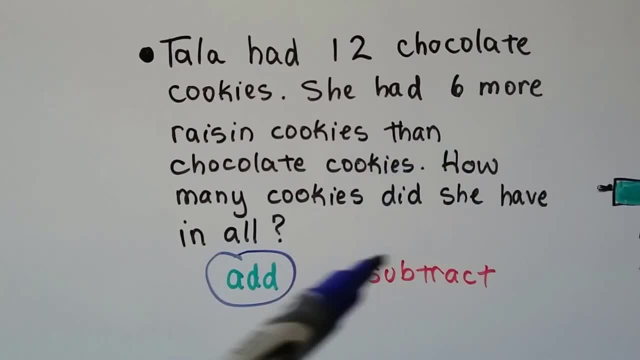 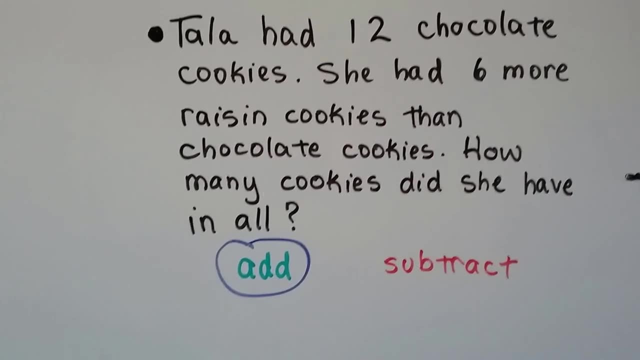 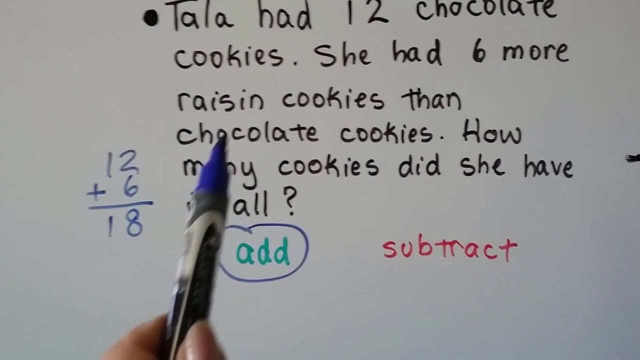 what that total sum is. Then we have to add it to the 12 to get the total amount of cookies she had. in all, 12 plus 6 is would be 18.. So that means she had 18 raisin cookies because she had 6 more. 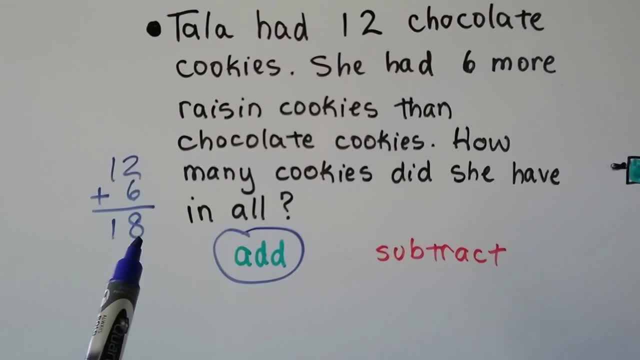 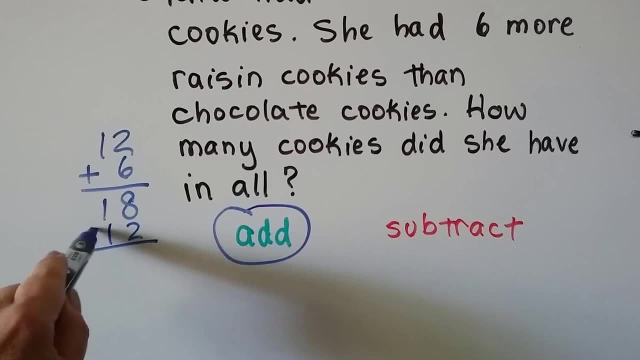 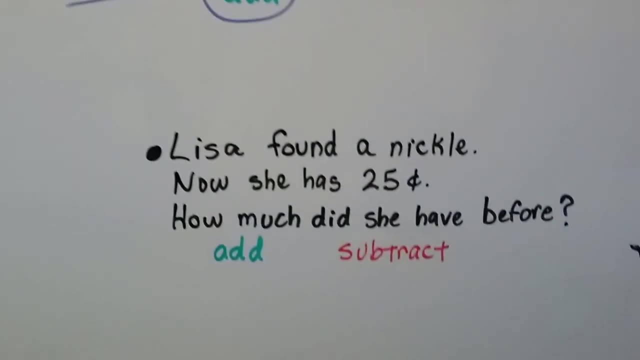 than the chocolate ones. How many did she have in all? Well, if 18 was raisin and 12 was chocolate, now we would have to add the 12 chocolate to this, See. So it's adding and then adding again. See Two parts. Lisa found a nickel. Now she has. 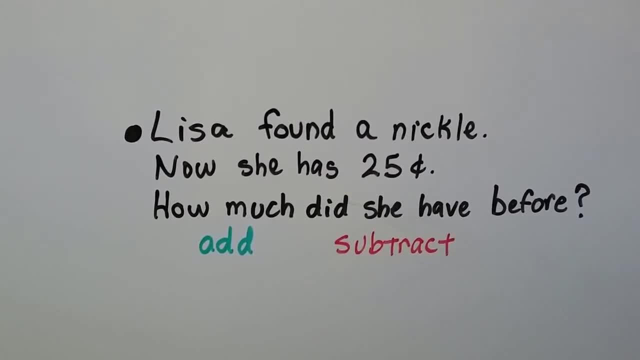 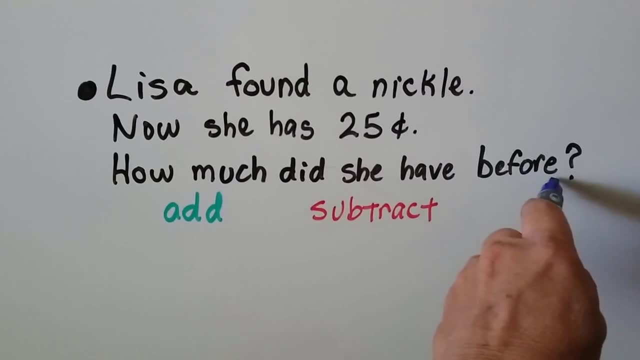 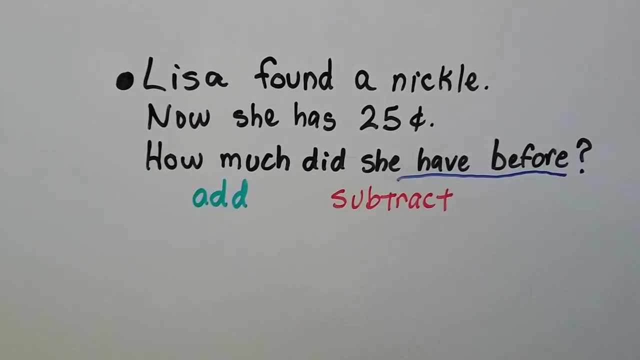 25 cents. How much did she have before? Would this be adding or subtracting? Well, this right here have before tells us that it was before she found the nickel. So that means we need to take the nickel away from the 25 cents to find out what she had before.